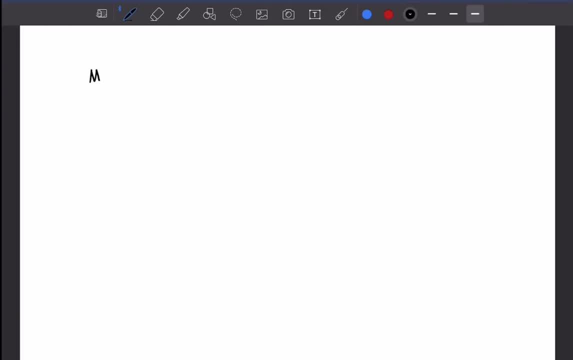 The differentiating factor between this is that if you, if you remember, you can see that the d-block and the f-block elements contain main group elements. So main group contain s and p-block elements. So these elements are generally sometimes metals. 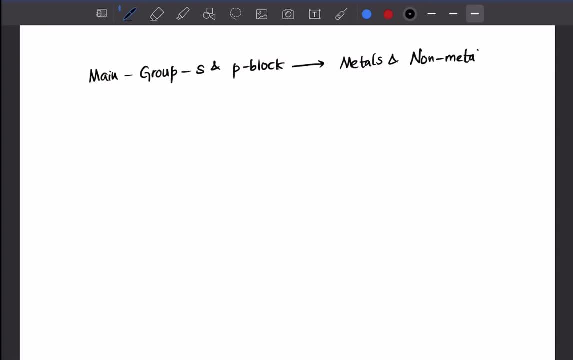 and sometimes non-metals, But when it comes to d-block and f-block elements, these are completely metals. So and one special group in f-block that there are two rows of elements. So the first row are called actinides. 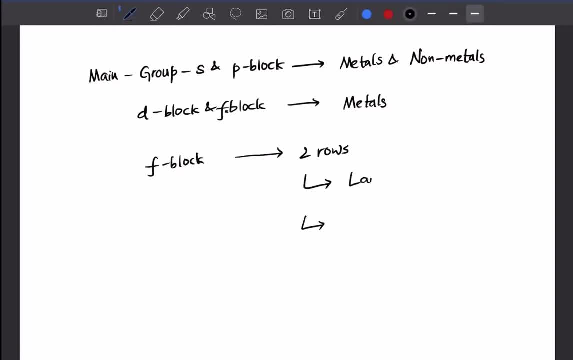 So the first row are called lanthanides And the second row are called actinides, So lanthanides, because they are the elements after lanthanum. Remember that lanthanum is not a d-block element, But elements after the lanthanum are called lanthanides. 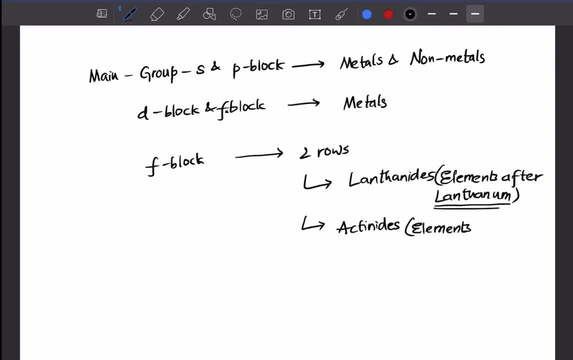 Actinides are elements after actinide actinum. So this actinium is also not a transition transition metal. So in d-block elements you will see multiple elements. So this is the biggest group of elements in transition elements. 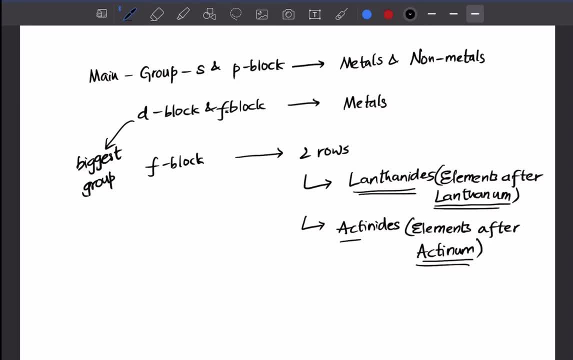 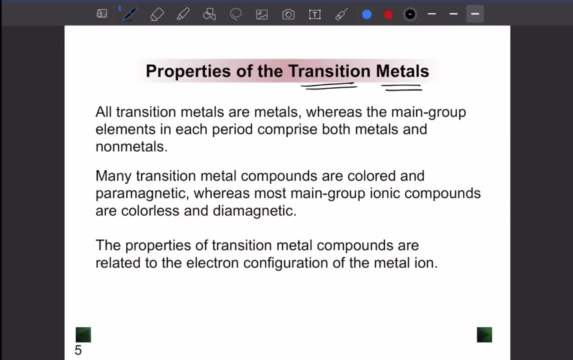 So we'll talk more about them as we go along, But remember lanthanides and actinides. What are the common properties of transition metals? So first property- we already discussed, We already said- is that all transition metals are metals. 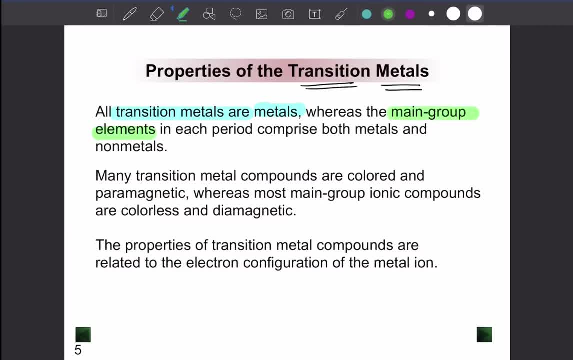 So, whereas main group elements can be metals and nonmetals. So because they can be metals and nonmetals, So the chances are they can be both at the same time. Now, many transition metals are generally colored compounds and they are generally paramagnetic. 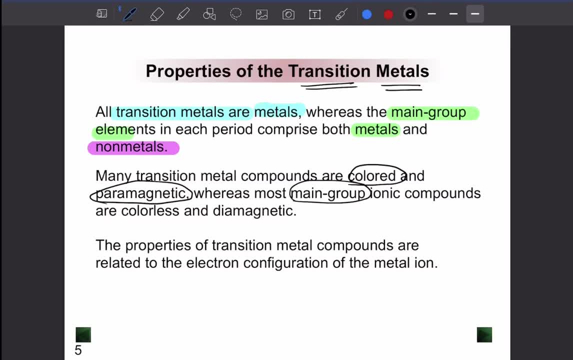 So, and most main group elements are generally ionic compounds that are colorless and diamagnetic. So again, the differentiation between paramagnetic and diamagnetic, So in paramagnetic is influenced slightly, So in paramagnetic it is influenced by magnetic fields. 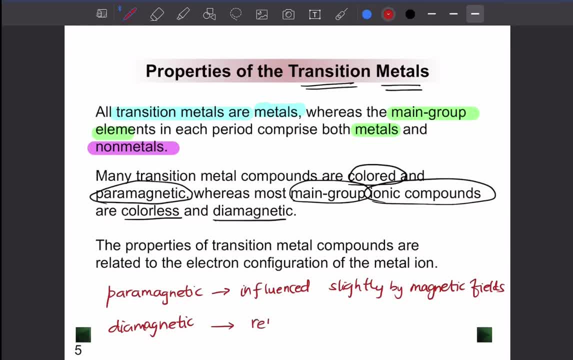 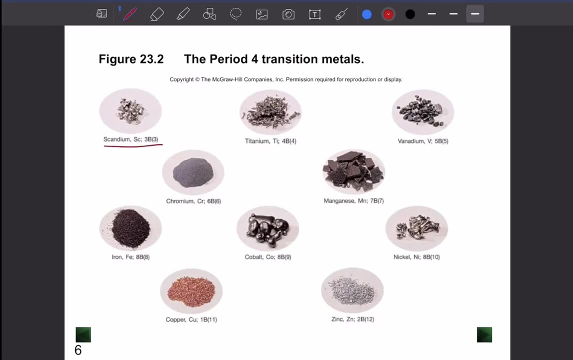 So diamagnetic substances are supposed to repel magnetic fields? They are supposed to repel magnetic fields, or you can simply think that they are not influenced by magnetic fields. So these are some elements. So these are some elements, For example, scanium. you can find it in Earth. 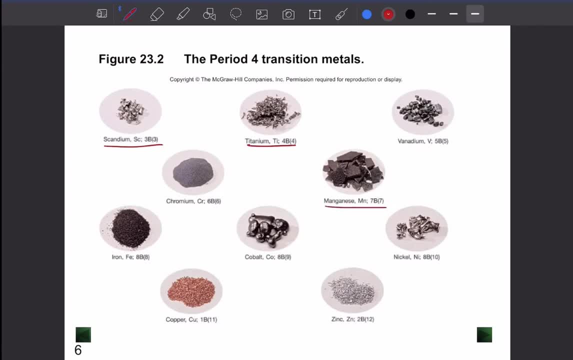 Titanium is another metal. Manganese is another metal we use. Cobalt is the element present in vitamin B12.. You can see nickel, zinc. Zinc is an element present in an element, an enzyme called zinc carbonase, An enzyme called zinc carbonase. 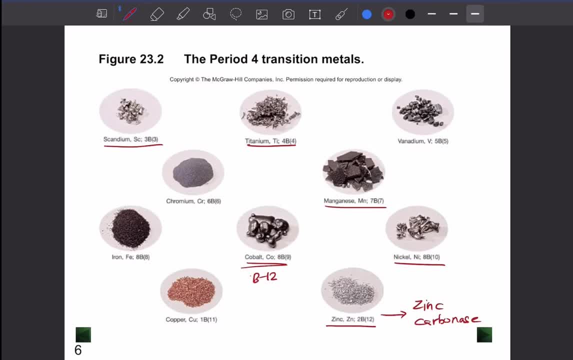 This is the enzyme that is used to remove carbon dioxide. So it is used to remove carbon dioxide. Fantastic, Excellent. So that is all. えーne approves Boutique. Goodbye, Bye, bye from your lungs. and you also have iron, chromium, copper and also vanadium. these 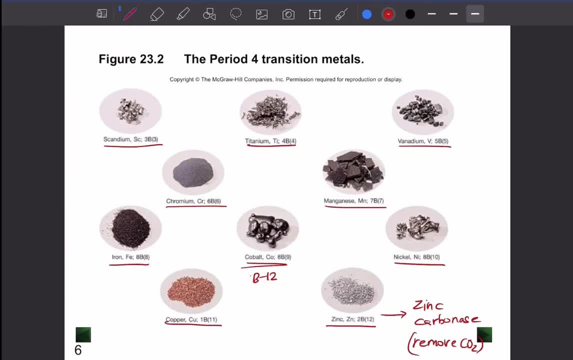 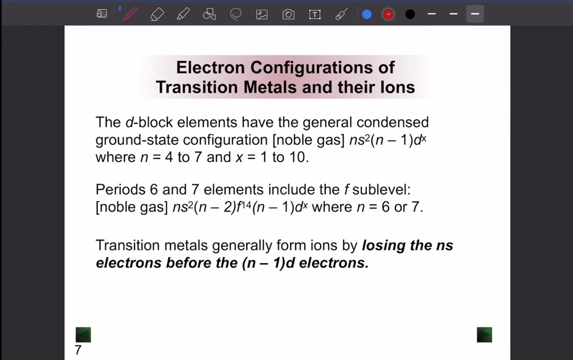 are common metals that you find in your body as well. some elements are generally found in the body, the. those elements are generally called essential metals or essential vitamins. we call them essential materials because they are needed for your body to function properly. so let's go to the next topic. 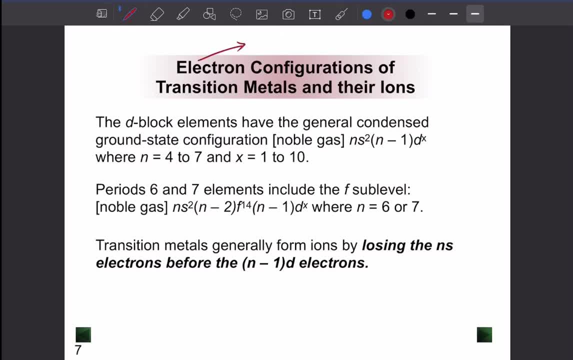 which is how do you calculate the electron configuration or how do you write the electronic configuration for transition metals? so d-block elements have a general condensed ground state configuration. so again, remember, ground state configuration are L configurations when they are not charged right. so the general configuration is ns2 n minus 1 DX. 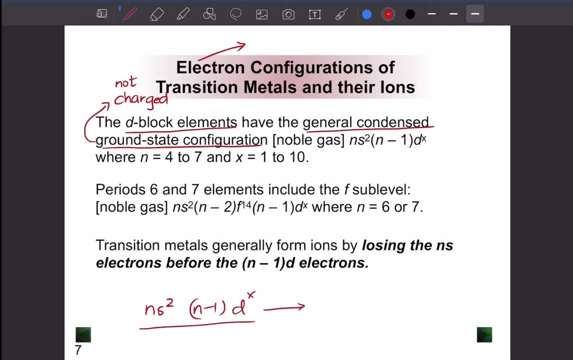 this is n minus 1 dx. this is n minus 1 dx, the general configuration for d-block elements you have. we have block elements. the general configuration is: ns2 n minus 2, f14 n minus 1 DX. this is the configuration, for you have block elements, so it's not exactly a block. 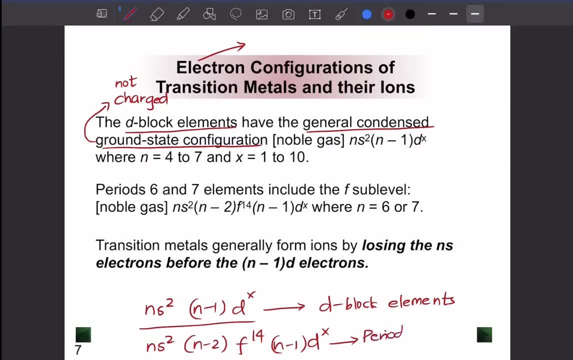 elements, but these are elements in period 6 and 7 of d-block elements. so and then you have block elements. you generally end up with ns2 n minus 2 fx. so this is the configuration for a block elements. one peculiar characteristic in transition metals is that transition metals before losing the d-sub shell is. 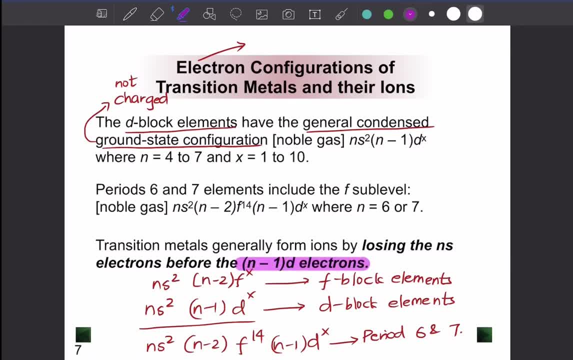 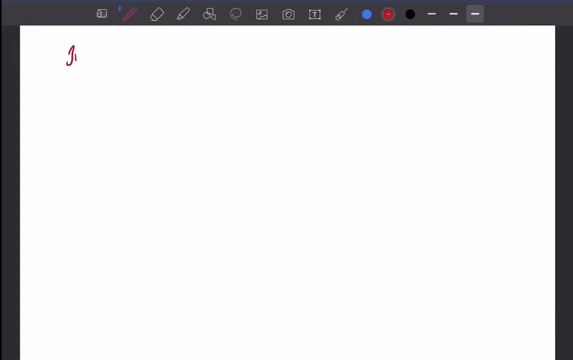 so before losing electrons from the d-sub shell they actually lose electrons from the ns2 sub shell. so the ns sub shell is the first one that loses electrons. so I'm going to emphasize this point again. so in d-block elements electrons are removed first in ns2 sub shell before the n minus 1 d-sub shell. so before the 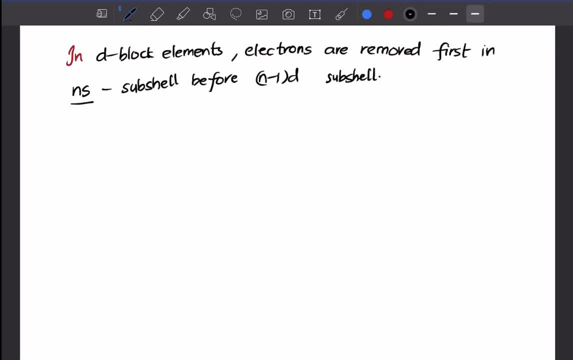 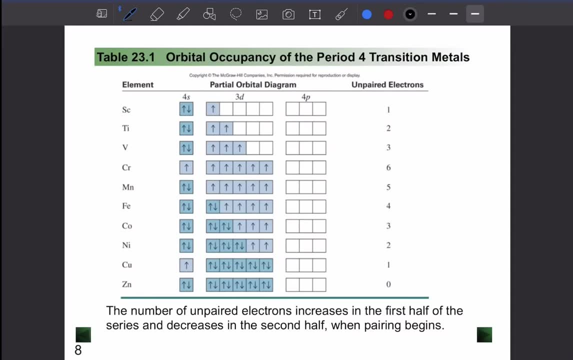 ns2 sub shell is first removed in ns2 and then, if there is anything more, then they are removed in n-1d now. so if you take an element of scandium, we talk about orbital occupancy. orbital occupancy is the rate at which the electrons are occupied in an element. so what do I mean? 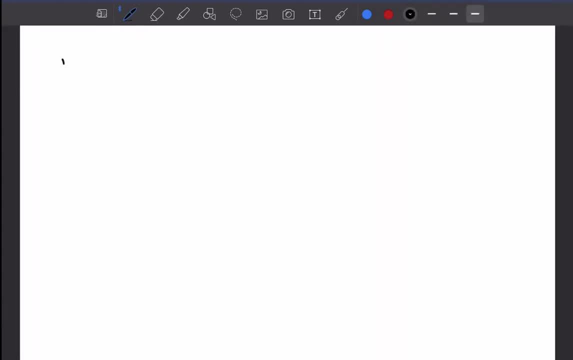 by that. if you take the first element, scandium, so scandium has an electronic configuration, a z of 21, so if you write down the configuration, the closest element is argon, which is 18, and then you get 3s2, and then you get 3s2, and then you get 3s2 and 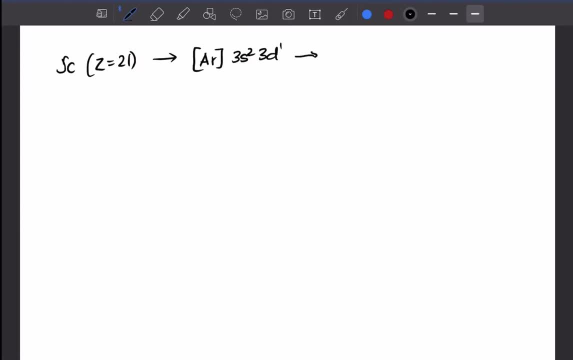 3d1. so when you write it in the orbital diagram, you have 3s, and then you have. so these are the orbital tables that you end up with. now, when you try to draw the number of electrons, so you get one, two, one, so that's three electrons. 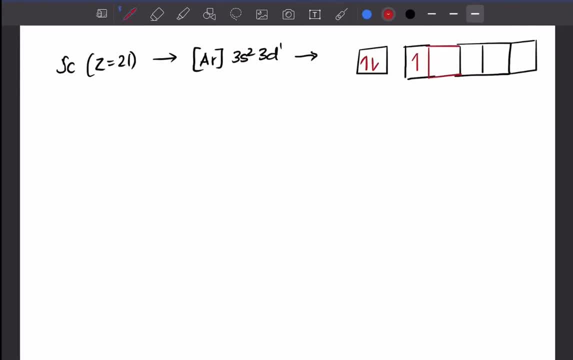 full. so this is for scandium. now, when you write it for the next element, titanium- titanium is that equal to 22. again you have argon 3s to 3d2. so when you write down the same table again. so let me copy this: 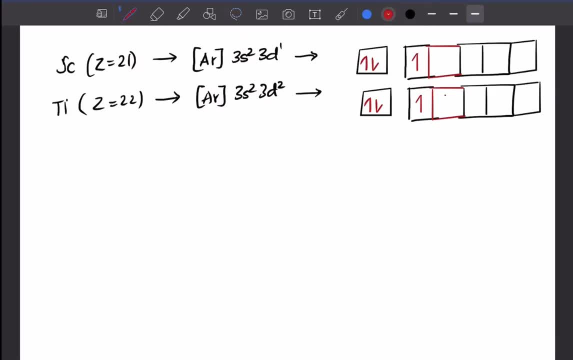 so we get two electrons in the d sub shell. so this is the s sub shell, this is the d sub shell. now we can continue writing this, but i want to focus on one main metal, two main metals: one is chromium and the other is copper. chromium has an atomic number of 24. 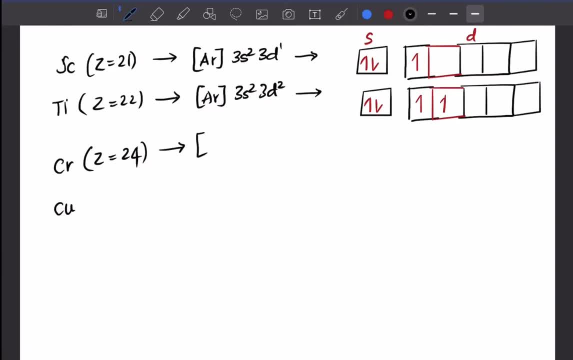 so when you write the electronic configuration it would generally be 3s2, 3d4. but the problem is that d likes to fill electrons before. yes, especially if it is close to half field. especially if it is close to half field, it likes to fill it before going to. 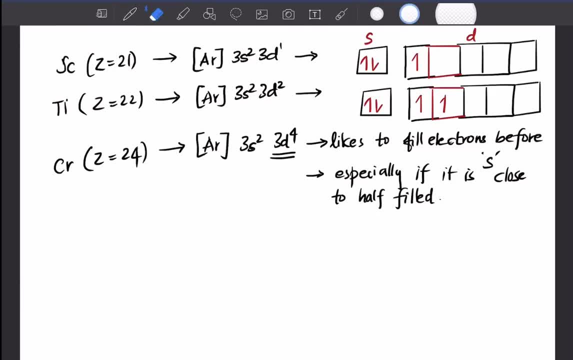 the s orbital. so what happens here? so, rather than the electron going directly into the d sub shell, the electronic configuration changes to organic argon 3s1 3d5, so it will fill up the d sub shell before it fills up the s sub shell. 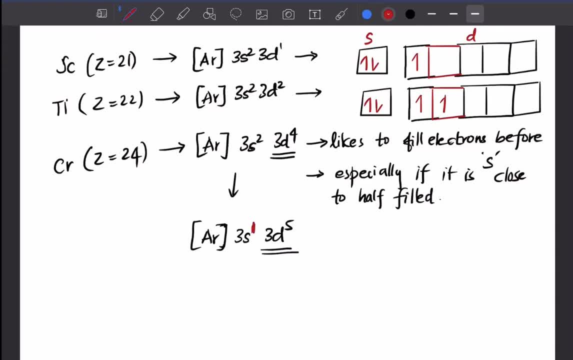 so focus on the s sub shell here. so there's only one electron here. so now, when you write the configuration, you get only one electron in the d sub shell. so one, two, three, four, five. this is one element where you will see that the argon, the chromium, 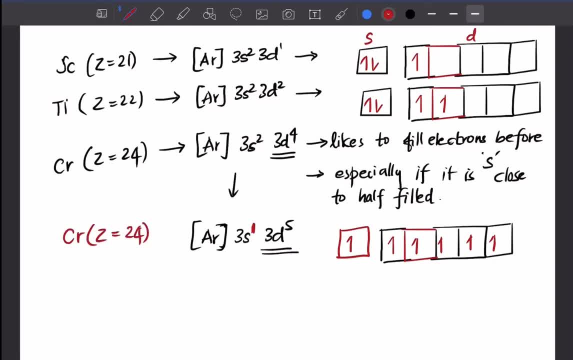 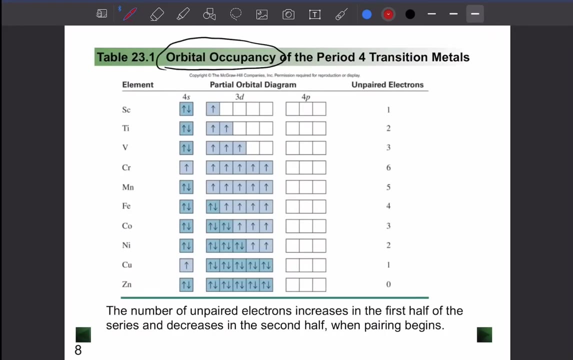 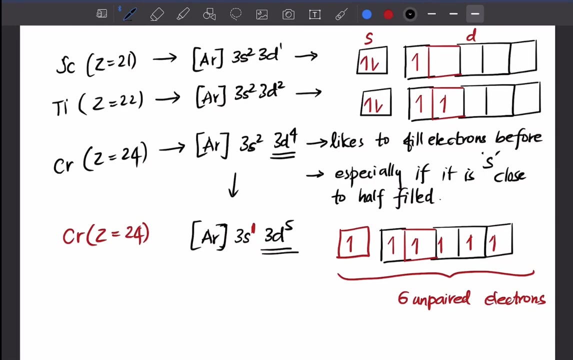 has. originally, if you look at it, it should have four unpaid electrons, but in originality it will have six unpaid electrons, so it will end up with having six unpaid electrons. now, another element that i want to focus on is copper, which has an atomic number of 29. so now, when you write the configuration, the original configuration- 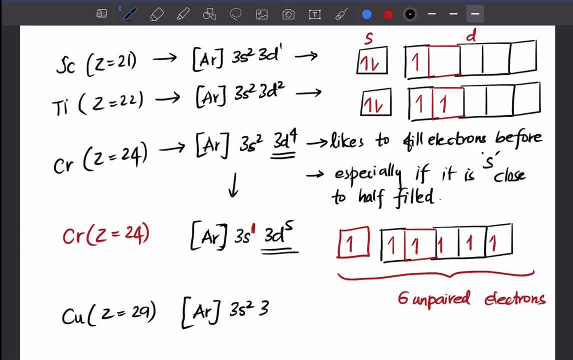 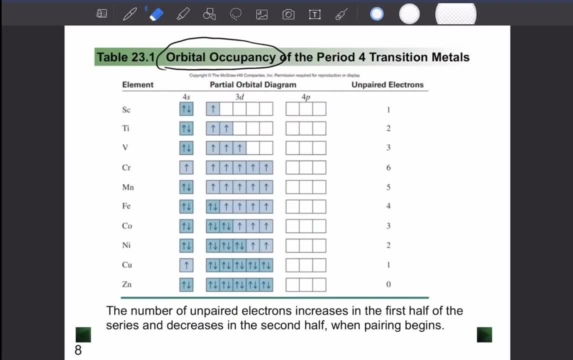 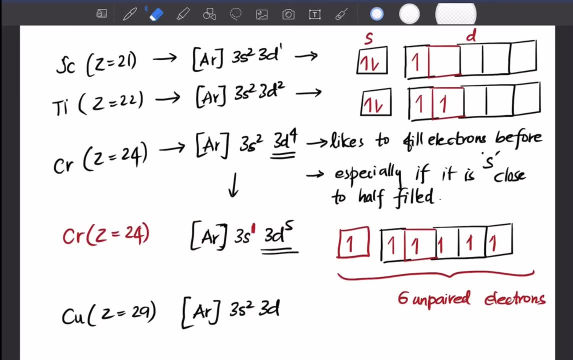 would be argon 3s to 3d9, but so so the configuration is argon 3d to 3d9, but it does not have. it has about only one electron left to fill in the orbital. so what happens is argon 3s to 3d9, but it has about only one electron left to fill in the orbital. so what happens is: 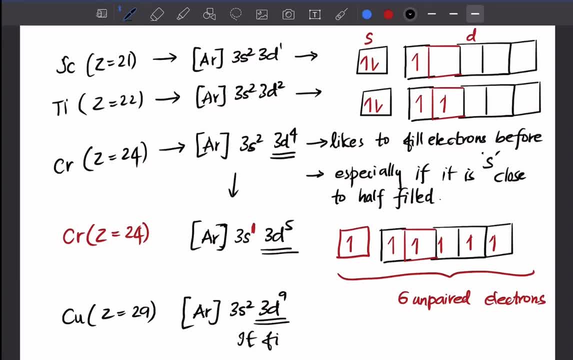 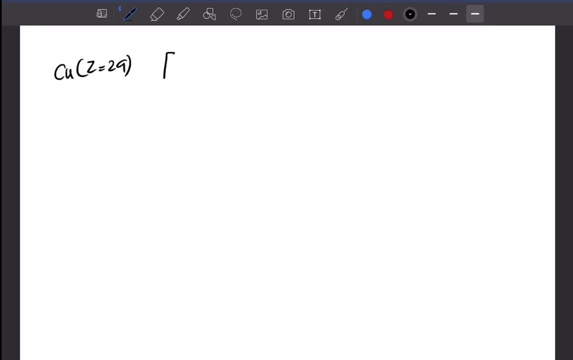 it fills the d orbital before the s orbital. so it fills the d orbital before the s orbital. so this ends up having an electronic configuration of copper z29 ends up having an electronic configuration of argon 3s1, 3d10. so now, so it will have one electron. it's the s suffering. 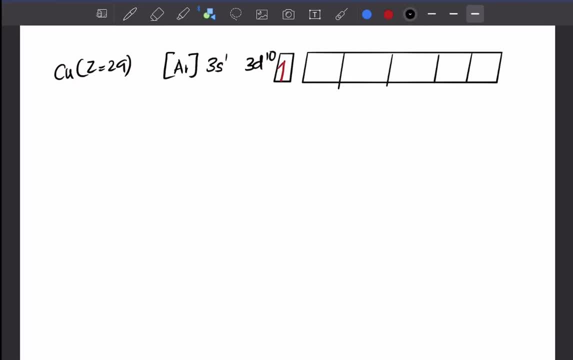 so one, two, three, four, five, and if you write out the number of electrons in the d subtial, you end up with a full orbital. so the idea here is: in copper the unpaired electron is in the yes sub shell. so the unpaired electron is in the yes sub shell, not in the D sub shell, as. 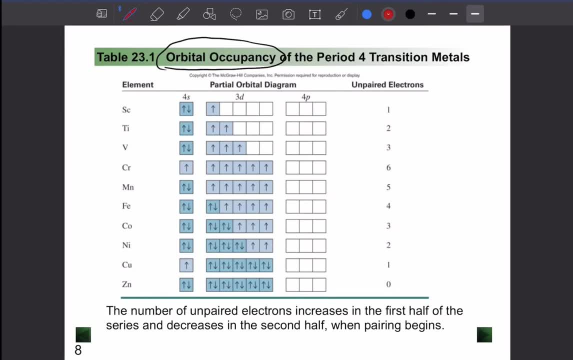 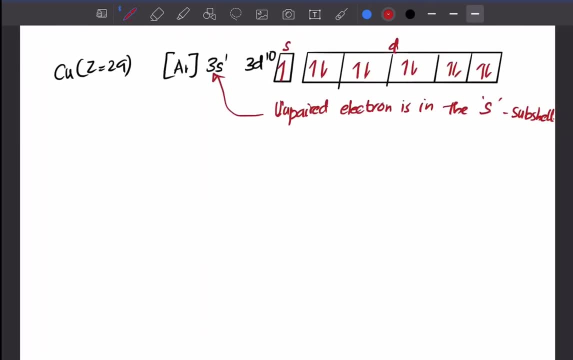 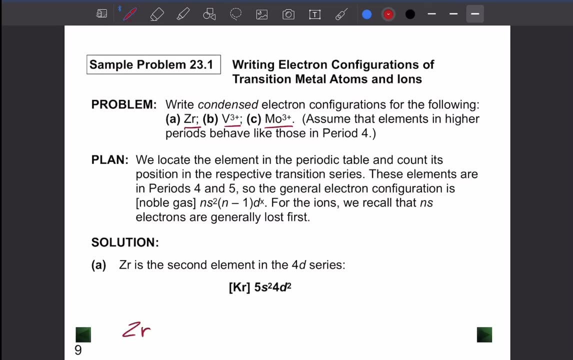 we think of. so this is the two peculiarities I want to notice in period four of the transition elements. now let's take an example of these materials and let's see one by one. let's take zirconium, so these are the three ones that you have: vanadium, three plus and molybdenum, three plus. so I'm 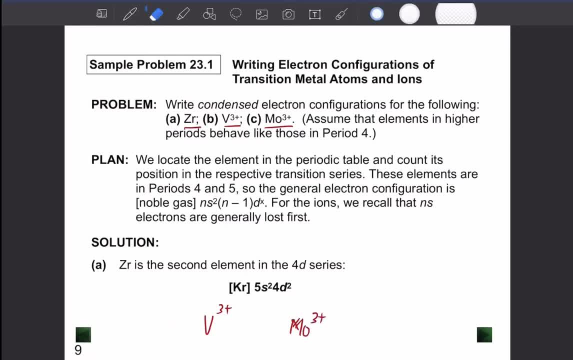 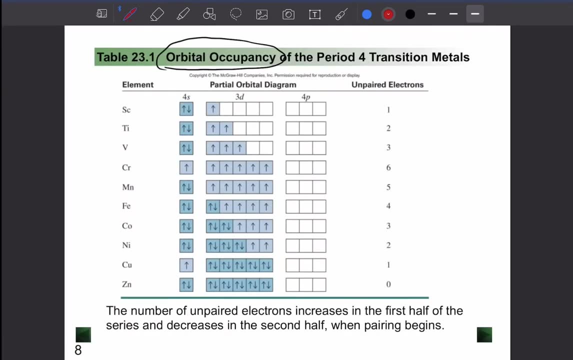 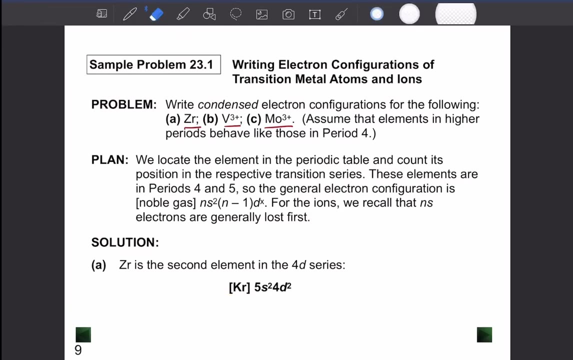 not gonna do zirconium. you have the answer here. try to do it on your own and find out the answer. so I'll do vanadium. so vanadium is the third element in the 3d series. so vanadium has vanadium of. it has an electronic configuration of. let me write it down. so vanadium has an. 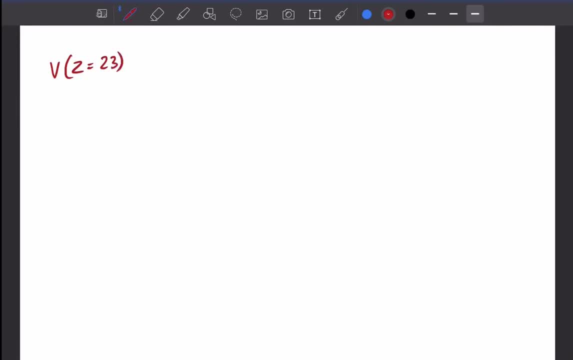 electronic number of 23. so when you write the electronic configuration you have argon 3s2, 3d3. so when you write the configuration, so you end up with the two electrons in the S shell and you have the D shell. so you have one, two, three, four. so you have one, two and three now. 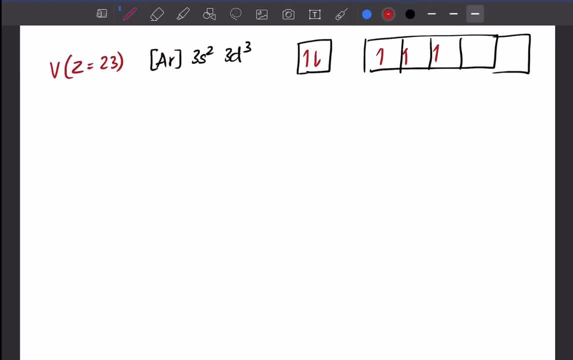 when you write the term vanadium three plus you will find out the two type of electrons which performed. so the question is: vanadium three plus. so whenever we write three plus it means that gets lost, loss of three electrons. plus represents loss of electrons, minus represents the gain of electrons. so this is in terms of the charge. now when we 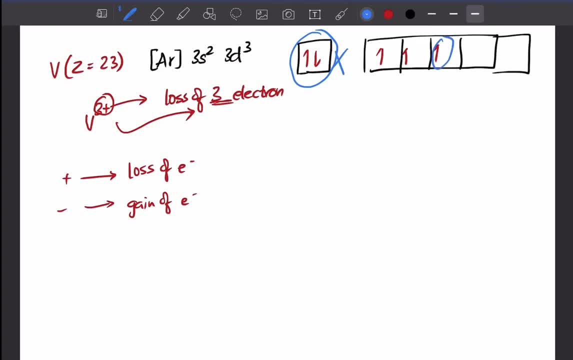 write vanadium three plus. where are the three electrons losing from? so the first, And then it goes to the D subshift. So when you write down the electronic configuration, you end up with argon 3D2.. So this is the electronic configuration. So benidium 3 plus. 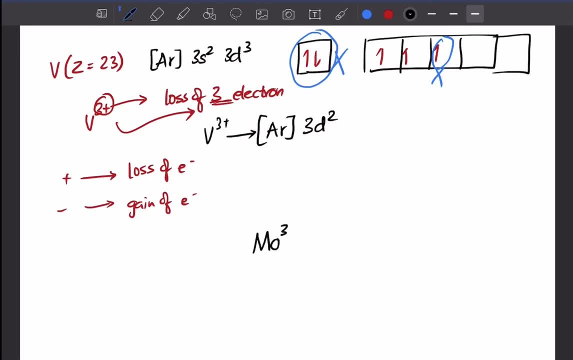 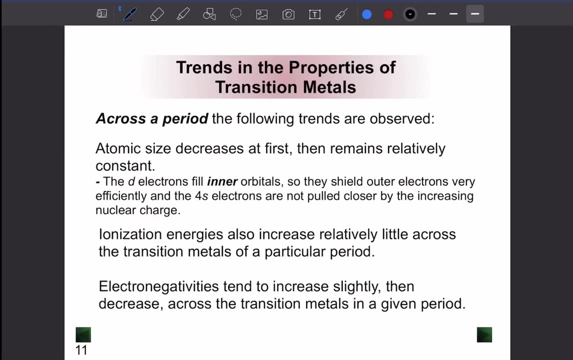 So pause the video right here and try for molybdenum 3 plus. So I hope you have the periodic table with you. So try for molybdenum 3 plus. What would be the electronic configuration? Next, what are the trends in the properties of the transition metals Across a period? these are the following trends that we generally observe. 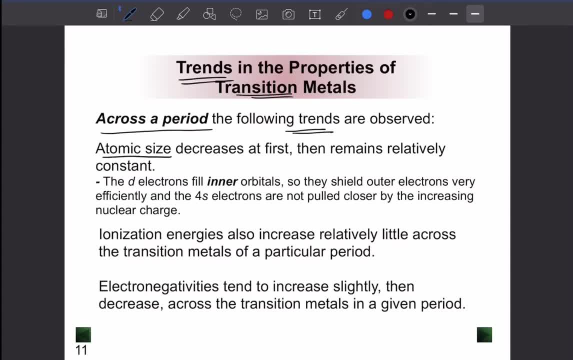 One is, the atomic size generally decreases at first and then remains relatively constant in the end of the table. So this is because The D electron fills the inner orbitals, So they shield the outer electrons efficiently. So then the forest electrons are not pulled closer by the increasing nuclear charge. 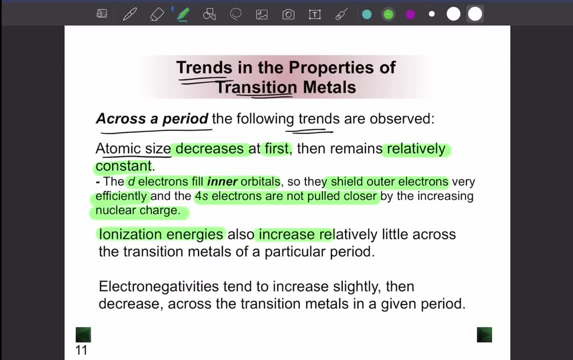 Next, ionization energies also increase because relatively little across the transition metals of a particular period, Electronegativities tend to increase slightly. Then they will decrease again across the transition metals. This is due to the stability. This is due to. 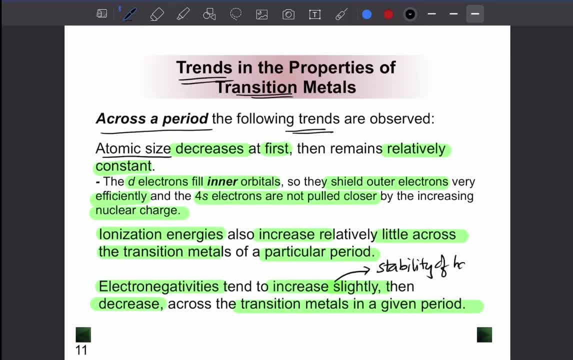 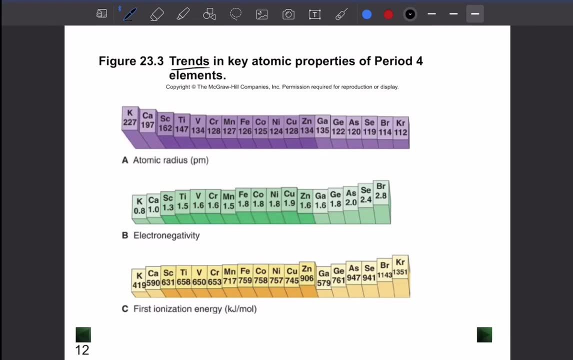 The stability Of half filled orbitals. This is due to the stability of half filled orbitals. Now what are the trends that we can generally observe? So these are the trends. So you notice that the atomic radius decreases slightly initially and then remains gradually nearly similar. 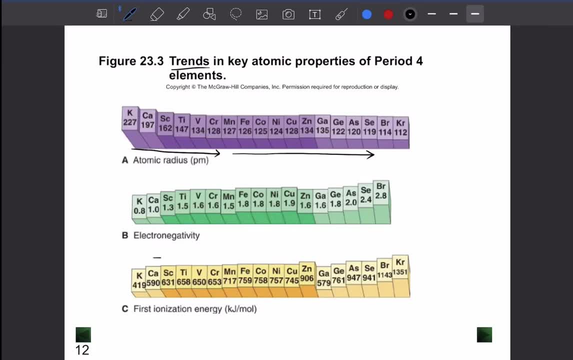 In electronic negativity. So if you look at the period table, it will increase slightly and then it will decrease again. so you will end up with a simple change here. so you have an increase and then a decrease and then another increase directly up. so there's the trend of the 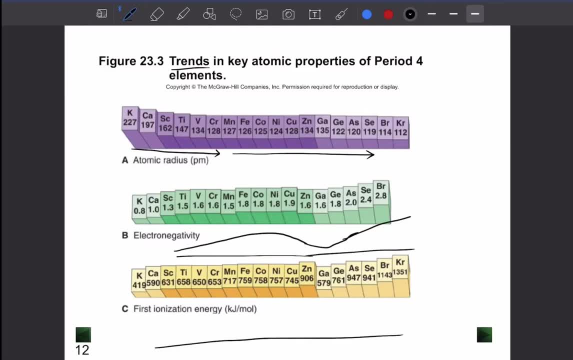 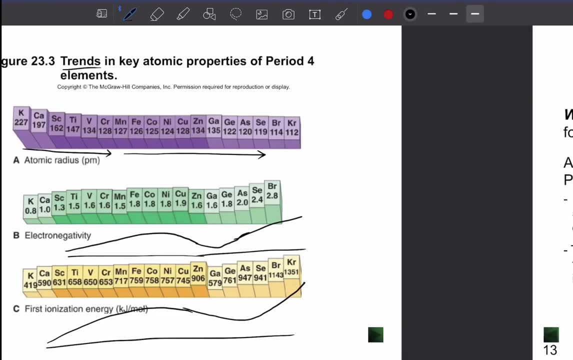 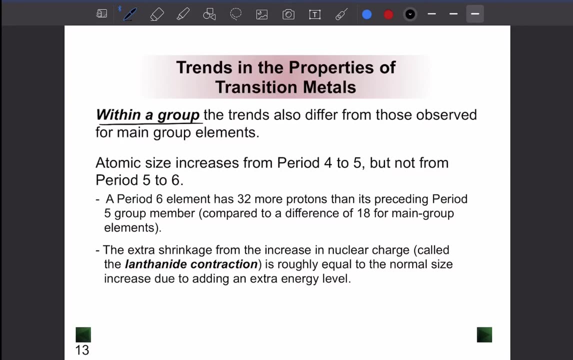 electronegativity. again the same with ionization: energy as you go across it increases rapidly and then decreases and then increases again. so this changes that are common, so one within a group, so the trends are also different from each group. so atomic size increases from period 4 to 5. 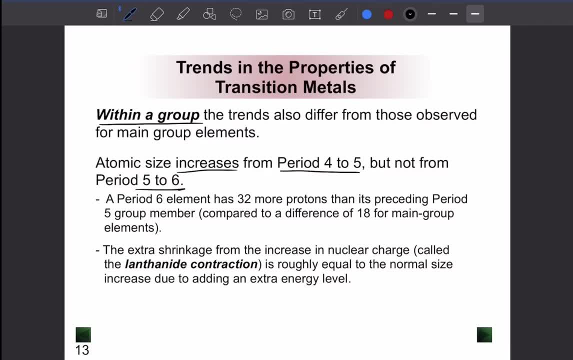 but from 5 to 6 it does not happen. this is due to a property called lanthanide contraction. so for period 6 and 7 elements. so for period 6 elements, it has 32 more protons than its preceding 5 membered. 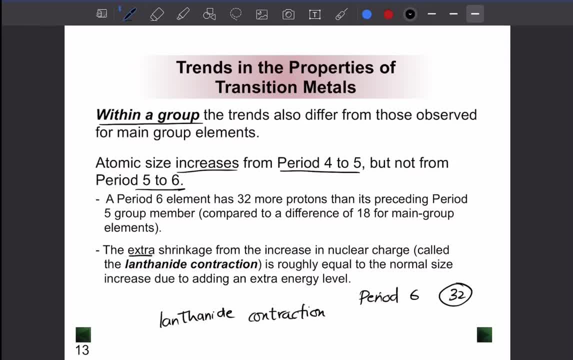 group. so what does that do? is that it increases the shrinkage and increases the nuclear charge and it becomes nearly equal to the normal size due to the extra energy level because of the presence of the F sub energy level that creates the lanthanide contraction. so it basically 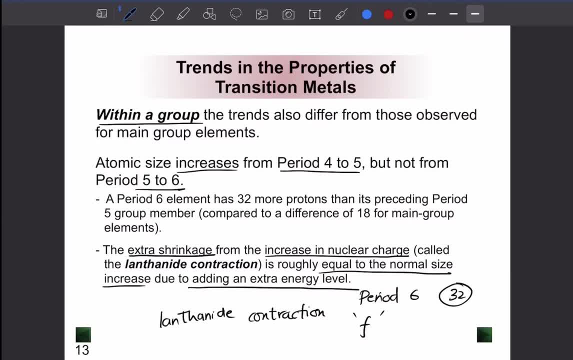 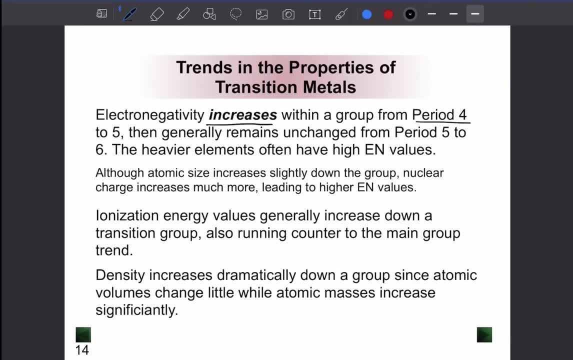 decreases in size because it's being pulled much closer because of the presence of extra protons. next, electronegativity trend also increases within a group from period 4 to 5, then generally remains unchanged from period 5 to 6 and, as the heavier elements generally have higher electronegativity values. 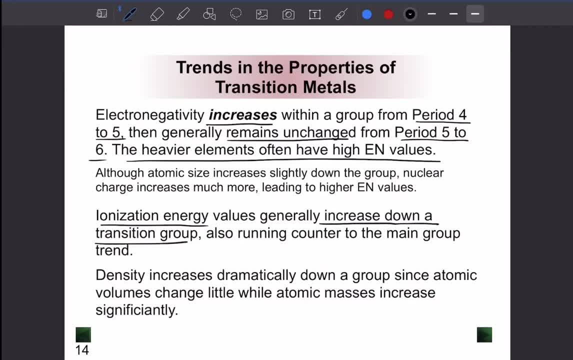 in terms of ionization energy the values generally increase down a transition group and also counter to the main group elements. so in main group element it generally decreases down a group. so ionization energy generally decreases down a group, but in transition elements it generally increases down a group. 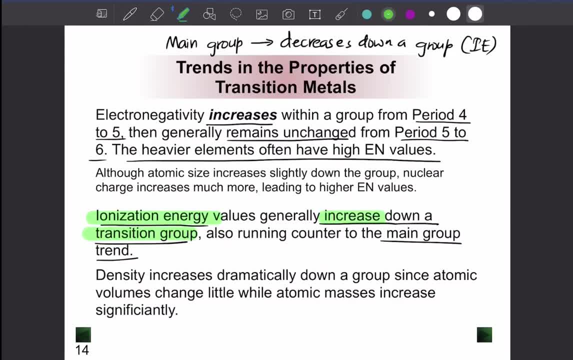 so ionization energy increases down a transition group, so density also increases dramatically. and then有沒有 of YO4 is reduced as respect to the rate of normal�를. it starts going down back again. so this dramatically down a group, since the atomic volumes here change very little, while the atomic masses increase. 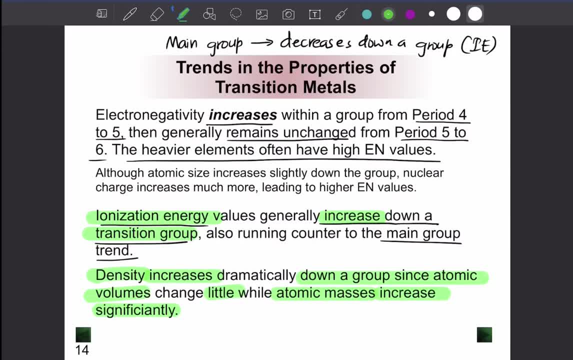 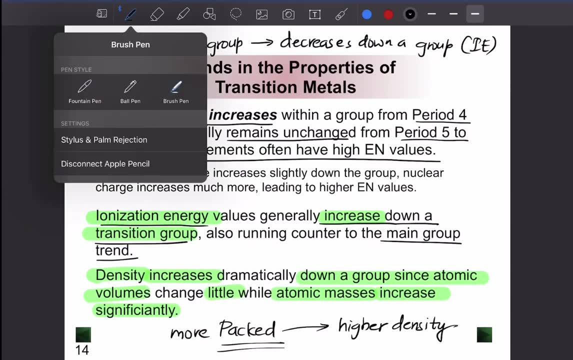 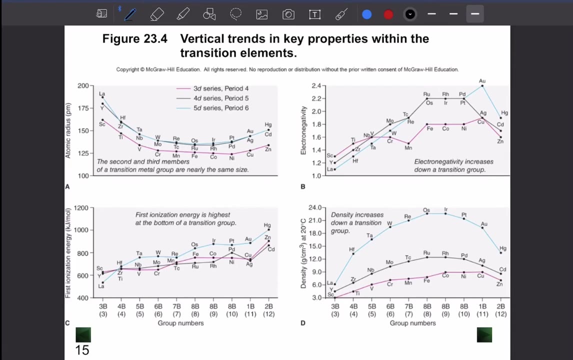 significantly, because they are much more packed, so the elements are much largely packed. so the more packed they are, the higher the density. so the more packed they are, the higher the density. so these are the graphs that explain the same phenomenon that I just told you about. next is oxidation states: most. 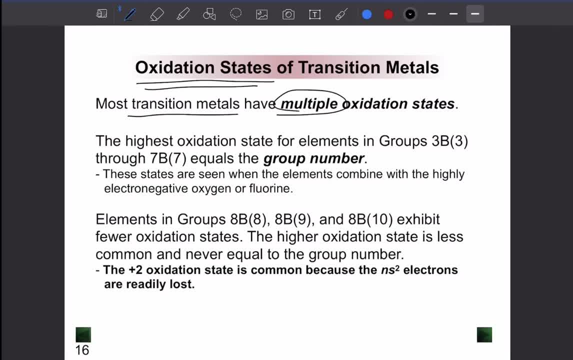 transition elements have multiple oxidation states. so the higher the oxidation element state of for the elements in group 3b- 2 through 7b- so that equals the group number. so if you have an oxidation state of 3 it means that it's a 3b group element. 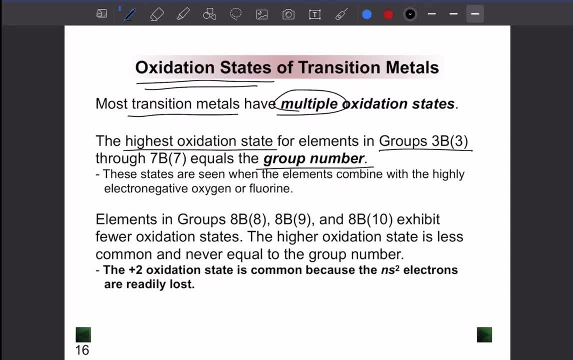 if you have an oxidation state of 7, it might be a 7b group element, but that only represents the highest one, so that's the limit to which maximum can happen. elements in group 8b- 8, group 8b 9 and 8b 10 exhibit fewer oxidation states. 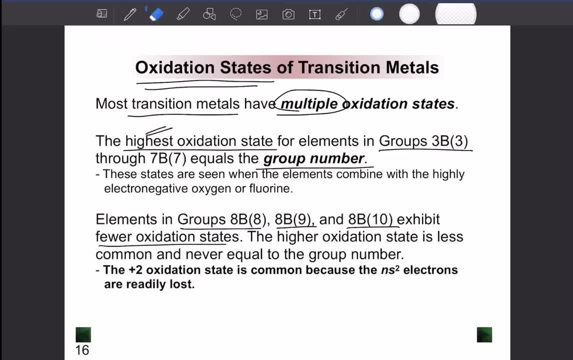 the reason is because the higher oxidation state is less common and never equal to the group number, only for 8b group elements, and the common oxidation state here is the plus 2 oxidation state. so best example of that is z n 2 plus. so z n is an 8b group 10 element, so 8b 10. 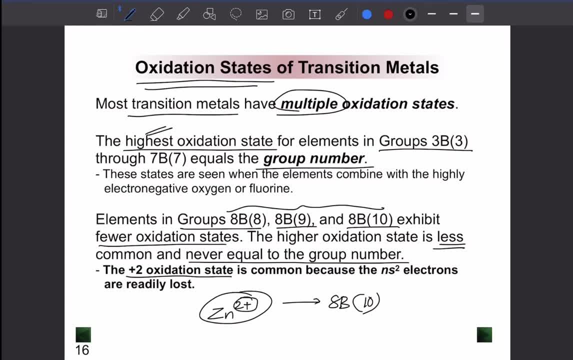 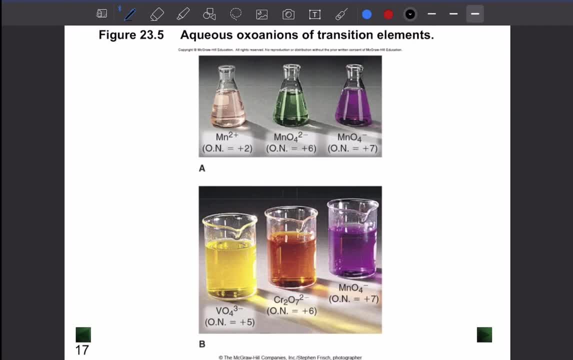 element. so if the common oxidation state that it can exhibit is 2 plus next. so these are some of the oxidation state from manganese. so manganese in MN n2 plus has an oxidation state of plus m, m, MNO4, manganese oxide 2 minus it has. 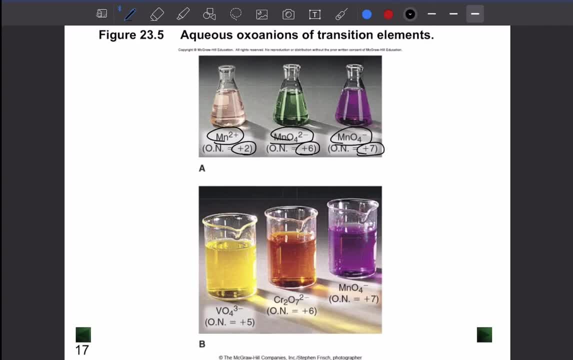 an oxidation state o plus 6 and Mno4 minus. it has an oxygen state of plus 7. Vanadium: it has plus 5, plus 6.. Chromium has plus 6.. Manganese has plus 7.. So these are some common anionic states. 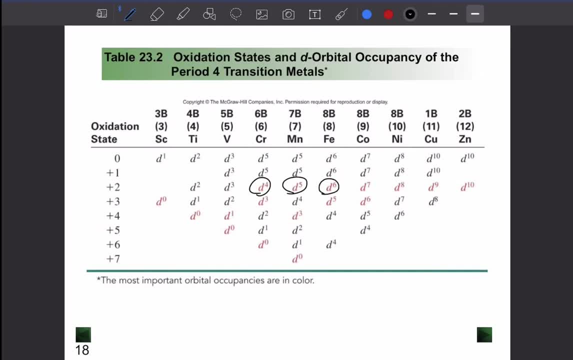 So the ones that you see in red are the common oxidation states. So one of the elements that has the common oxidation, the highest number of oxidation states, if you look at these, are the reds. these are the stable ones. So, if you look at the elements, the common one that has more number of oxidation states than the other is manganese. 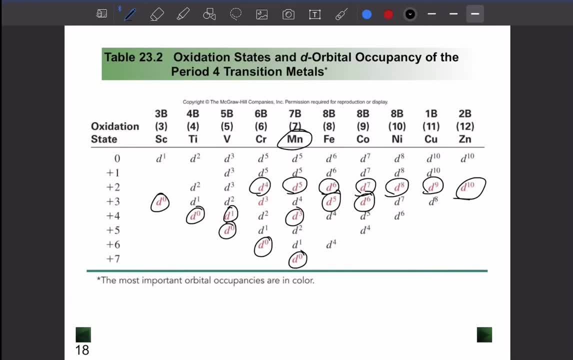 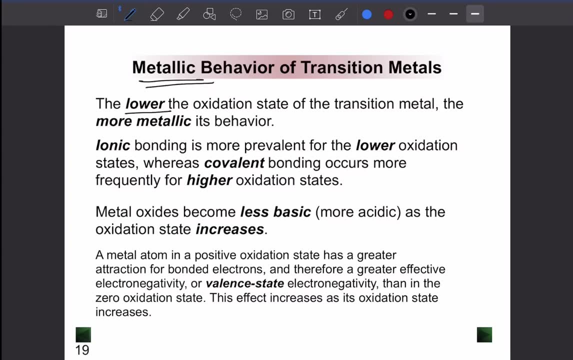 So manganese has the highest number of oxidation states present in it. So in terms of the metallic behavior, the lower the oxidation state, the more metallic its behavior. So ionic bonding is more prevalent when you have a lower oxidation state, whereas covalent bonding is common when you have a higher oxidation state. 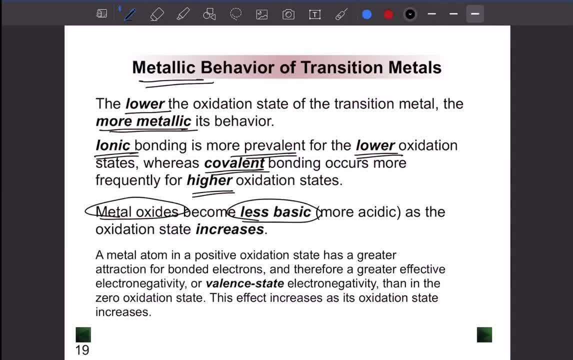 So in the same way, metal oxides become less basic when you have a larger oxidation state, So it becomes more acidic. basically, when you have oxidation state, So when the oxidation number or the oxidation state starts increasing, so the acidic behavior also starts increasing. 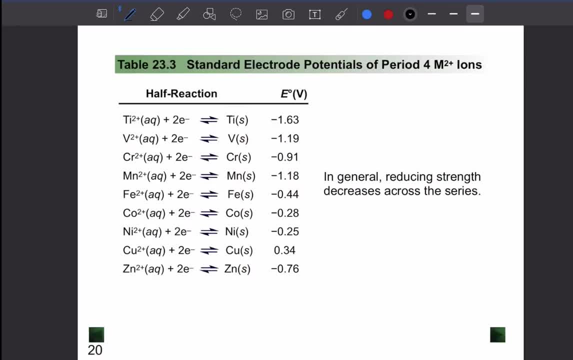 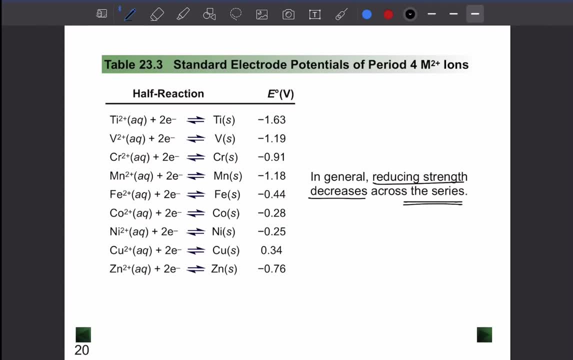 This is the metallic behavior of transition elements. So, and also one other one is the reducing strength also decreases across the series If you look at period. So in period four elements, so in period four, across the period. the value starts decreasing as you go down the period. 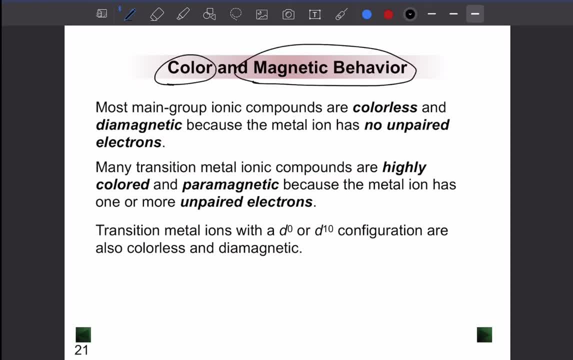 Next is the color and the magnetic behavior. So most main group elements are generally colorless and diamagnetic materials because the metal has no unpaired electrons. So one main group that can help in understanding magnetic behavior is the presence of unpaired electrons. So when you have unpaired electrons you both get color as well as some magnetic behavior. 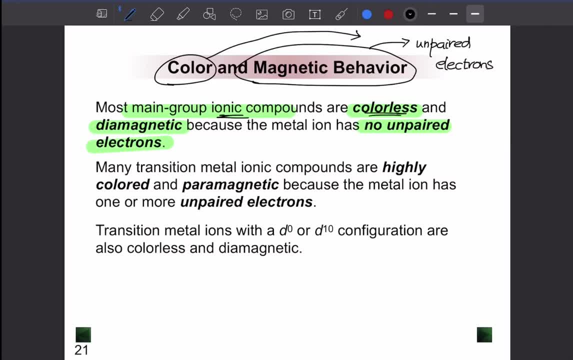 So most ionic elements are generally colorless. For example, the best example of it is salt. Salt is a colorless crystal, So if you take some salts they are pink. Those are generally made of some kind of a transition element. 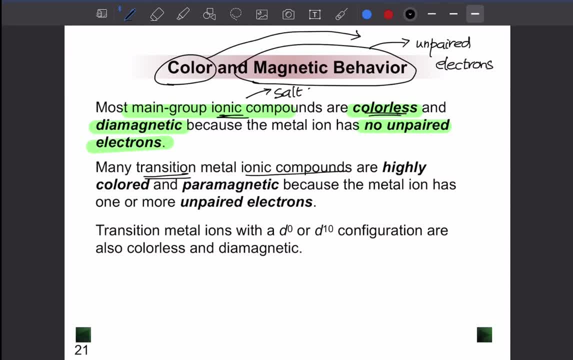 Next, if you have many transition, ionic compounds are generally highly colored and they are generally paramagnetic because they at least have one or more unpaired electrons. So the higher the number of unpaired electrons, the more the metallic behavior, the more the magnetic behavior of the substance. 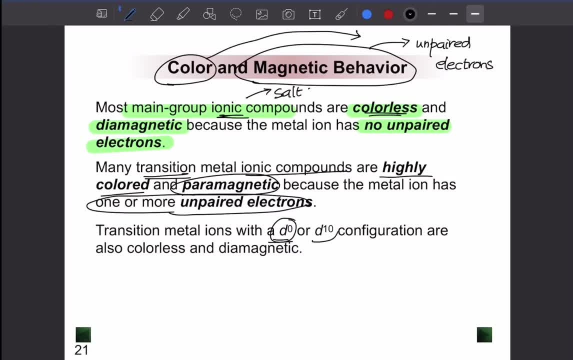 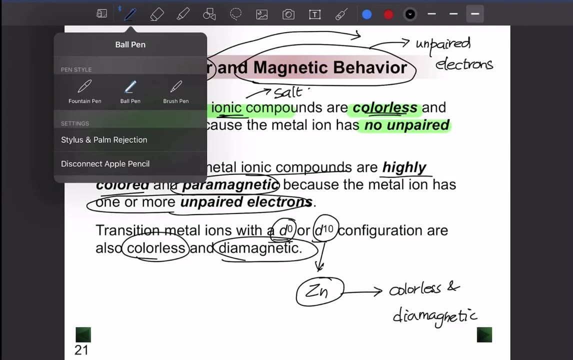 So transition metals with D0 and D10 configuration are also colorless and diamagnetic. One example of this would be zinc. So zinc in its uncharged state is generally a colorless metal And also diamagnetic. So what is generally done to increase its ability is we end up using zinc. 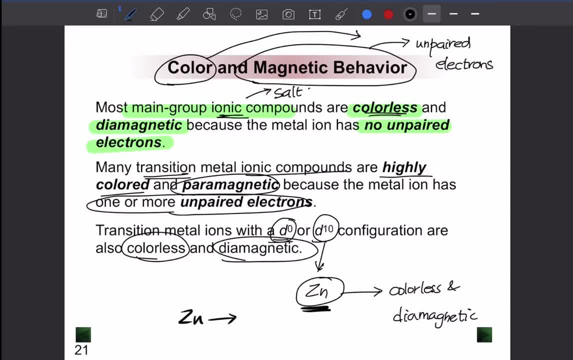 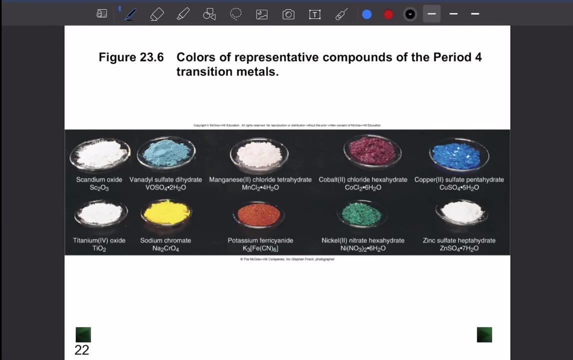 So we end up using Zn to find out whether we make it a charged metal so that it can become paramagnetic, It can become color, It can gain some color. So these are some elements and there are some compounds that they form and different colors. 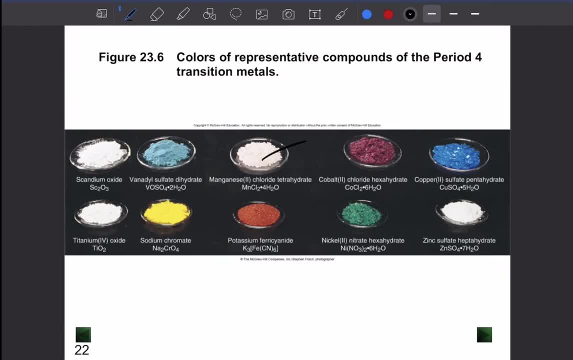 So notice that most materials have some colors, So notice the different colors that they can form. So one peculiar one, main one to remember, is for copper sulfate. Copper sulfate is generally a bluish color. Cobalt chloride hexahydrate is also a reddish color. 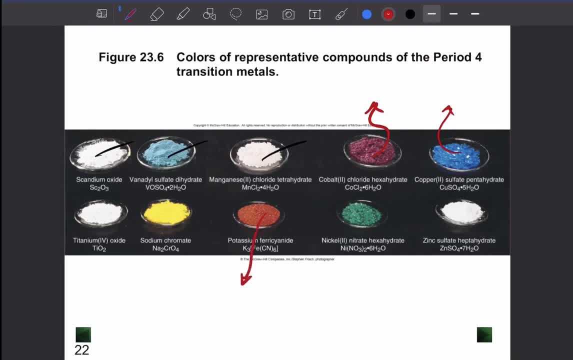 Potassium ferricyanide is also a reddish color. Sodium chromate is a yellowish material And zinc sulfate is a colorless material. The reason mainly is because it has it is in its uncharged or the uncharged state. 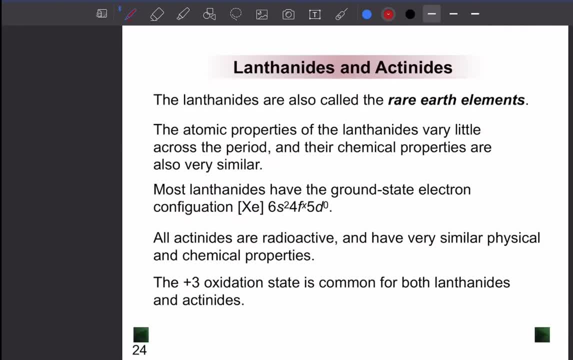 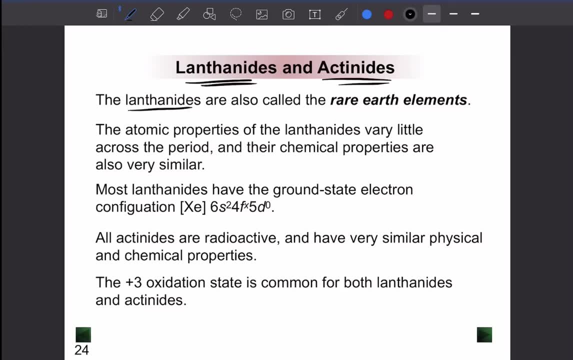 Now let's go to F block elements and lanthanides and actinides. So lanthanides are also called rare earth elements, Because these are rarely found in the atmosphere, In the earth's core, And they are found in very little amounts. 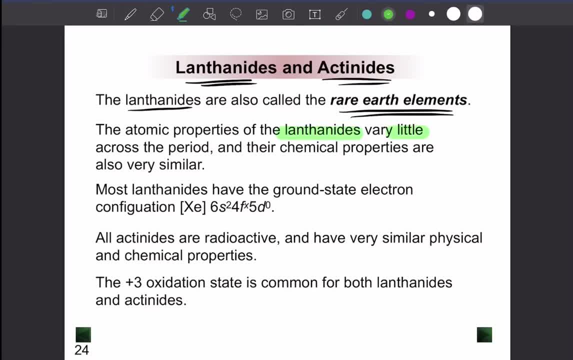 So the atomic properties of lanthanides very, very little across the period And their chemical properties are also really similar. So most lanthanides have the ground state configuration of xenon 6s2,, 4fx, 5d0.. 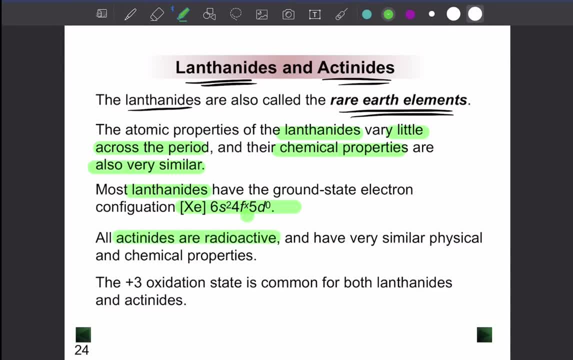 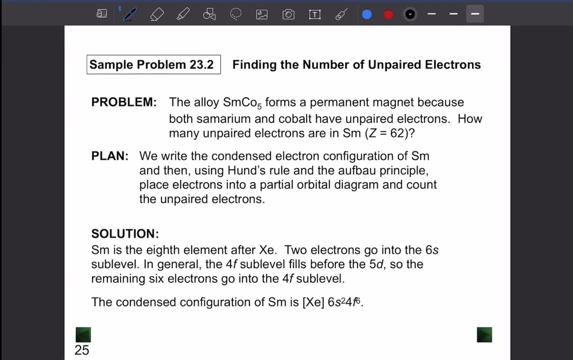 And all actinides are generally radioactive And they have very similar physical and chemical properties, And for both lanthanides and actinides the common oxidation state is plus 3.. So plus 3 is the common oxidation state found for both lanthanides and actinides. 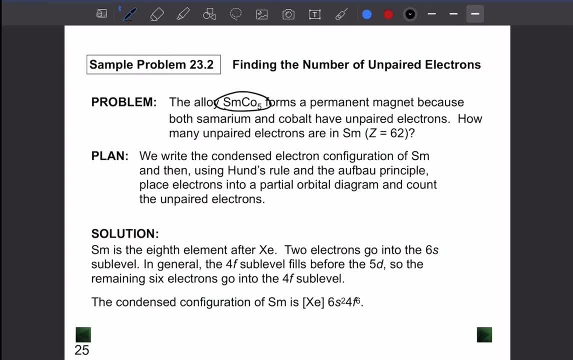 So let's take an example of smarconium. So smarconium is the fifth, eighth element after xenon. So you have xenon. The configuration becomes xenon 6s2, 4f6.. So, remember, the configuration is the noble gas. 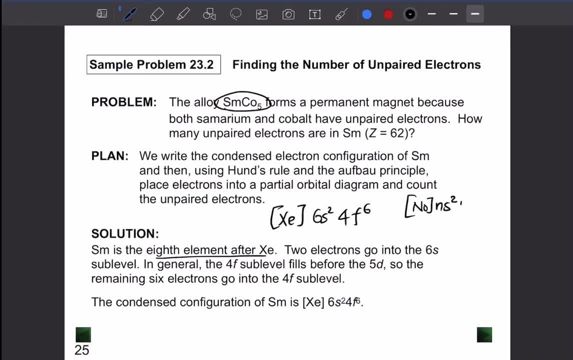 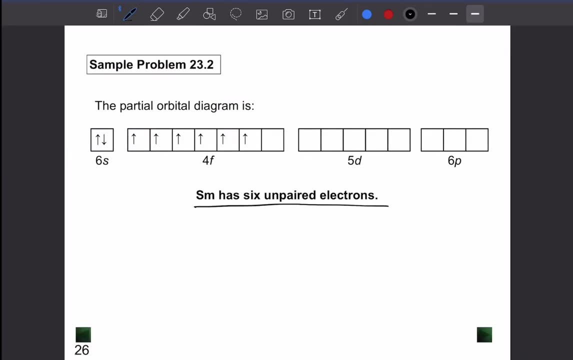 And you have ns2.. You have n-2, fx. So this is the common configuration that we generally find. So if you apply it here we get xenon 6s2, 4f6.. And so smarconium here has six anti-unpaired electrons. 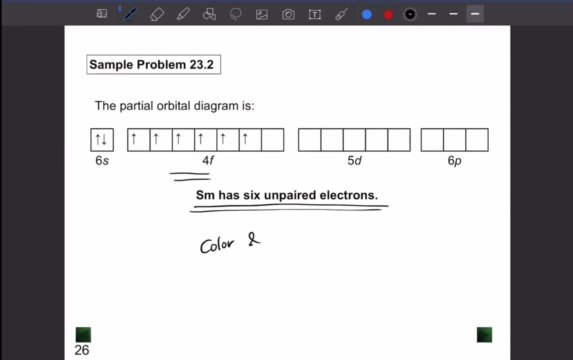 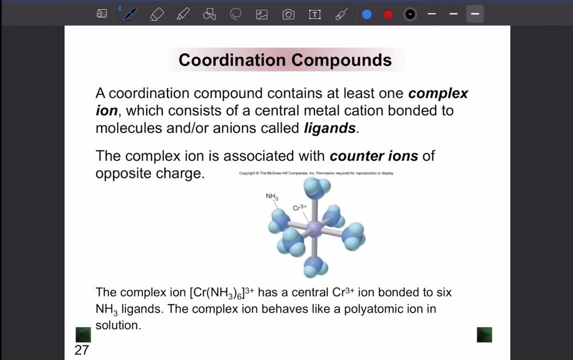 So it becomes: it's a color, it has color And it is paramagnetic. Now let's come to the main topic in this chapter: Coordination compounds. What is a coordination compound? A coordination compound is something that contains one complex ion. 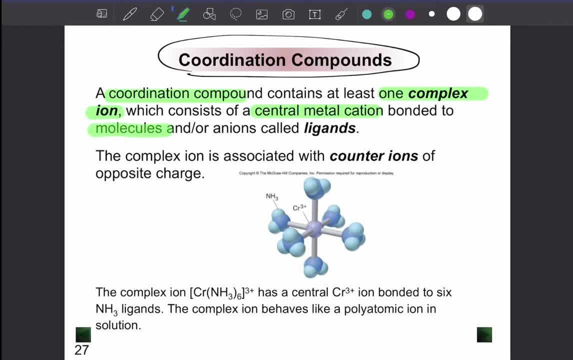 Which generally consists of a metal cation bonded to molecules or anions, And these molecules are called ligands. So whenever you see a ligand, it generally is bonded to something. It generally is bonded to something. So that's what we call a general ligand. 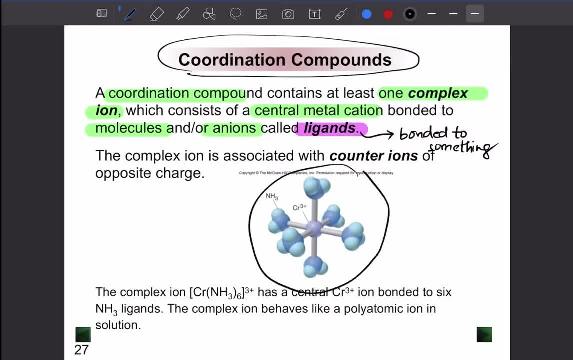 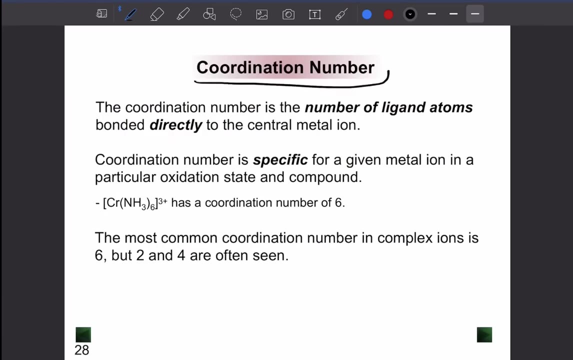 Now, the best example of this is this compound So, which is chromium NH3, taken 6, 3+. This is an example of this is an example of a coordination compound. Now We represent different coordination compounds with a coordination number. 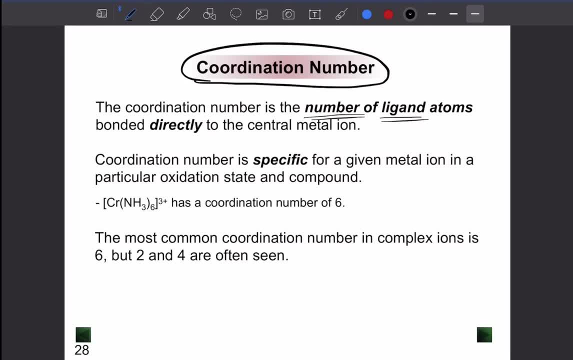 Coordination number is the number of ligand atoms that are bonded directly to the central metal ion. So coordination number is specific for every given metal And that generally comes from a particular oxidation state and compound. For example, the compound that we just saw has a coordination number of 6.. 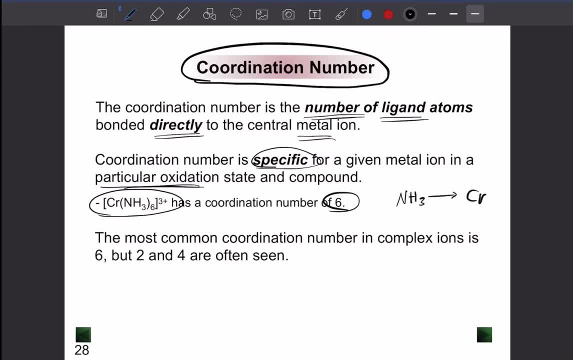 Notice that all the NH3s are connected directly to chromium And there are six of them. So we have that becomes your coordination number. The common coordination numbers are generally even numbers And they are generally 6,, 2, and 4.. 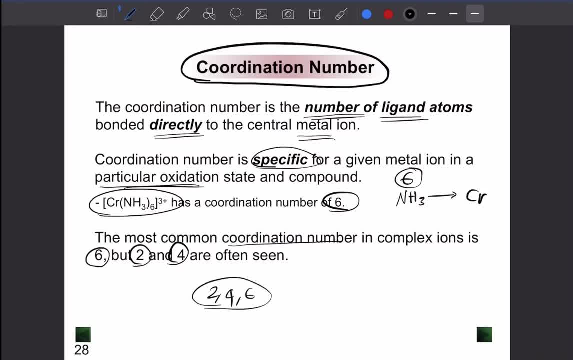 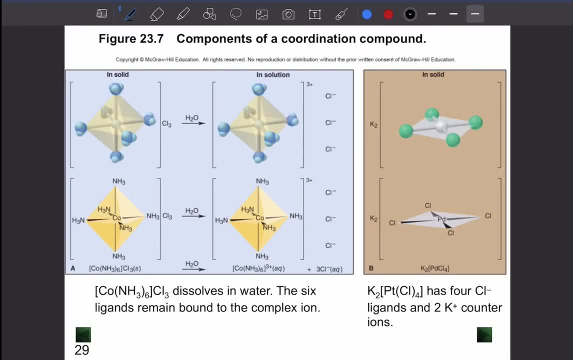 So you have 2,, 4, and 6.. These are the common coordination numbers that are generally seen. Now, what are the components of a coordination number? So coordination number contains a solidic material And something that dissolves in a solution. 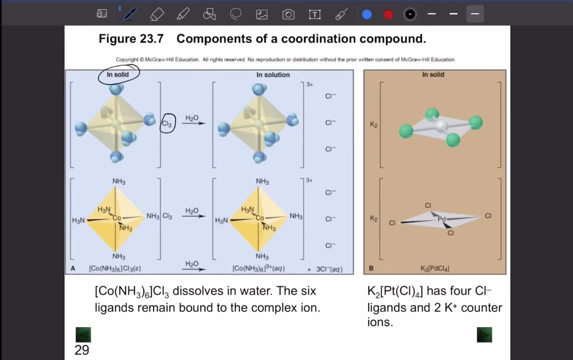 So how do you differentiate it? So when you dissolve it in water, it loses the charged material And the metal solution compound. it stays intact. That is what is called as the complex ion. So it makes an ion where one of them is really complex. 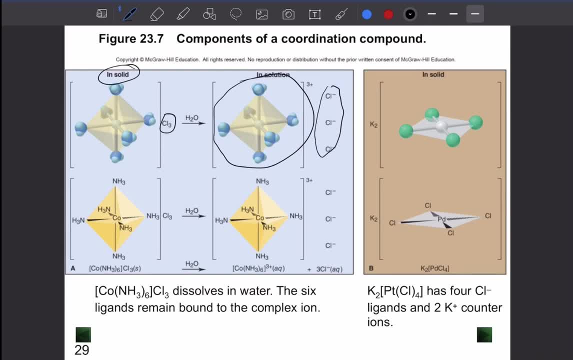 And it is bonded to simple ions, For example cobalt. this element here, CONH3, taken 6, Cl3.. When you dissolve it in water forms: CONH3, taken 6, 3+ plus 3Cl-. 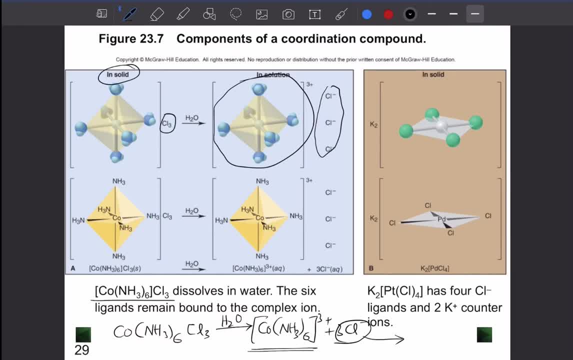 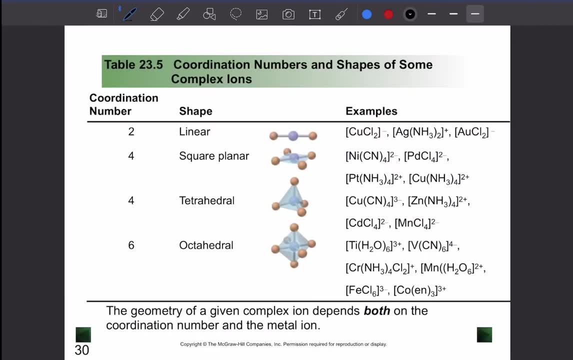 So 3Cl- becomes the simple ion. This compound is the complex ion. That compound is the complex ion. There are three common shapes, four common shapes that are formed with each coordination number. So for coordination number of 2, the common state is linear. 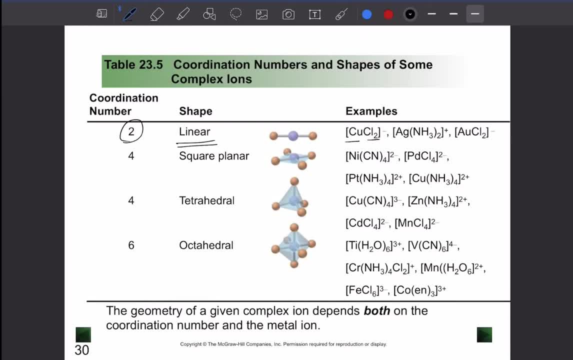 Where you have two elements that are directly bonded to the coordination compound And you have square planar, which is the coordination number of 4.. It has a plate shape, basically a square shape, Where you have a central metal ion and four of the ligands that are connected to it. 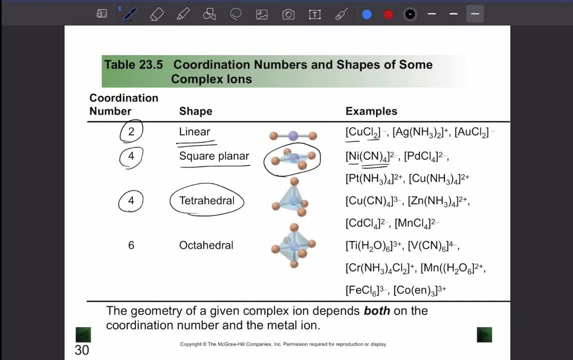 And another shape is a tetrahedral structure. Tetrahedral is a common structure that you have seen already. So you have again the four compounds that are connected to the central metal ion. We will see what conditions it becomes square planar. We will see what conditions it becomes tetrahedral. 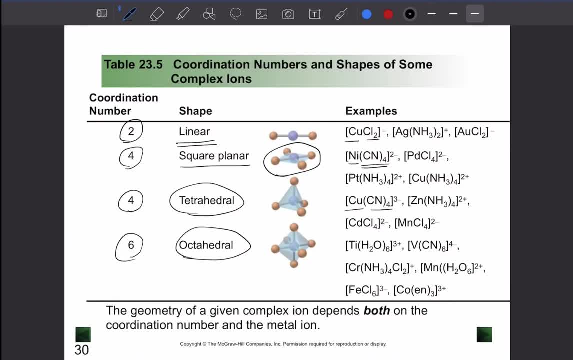 And if you have six of them that becomes octahedral. Octahedral is basically a simple construction of a rhombus. So if you connect all the compounds you get a rhombus. So that structure is generally called octahedral. 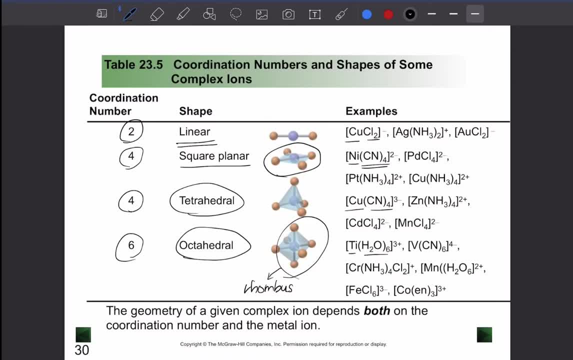 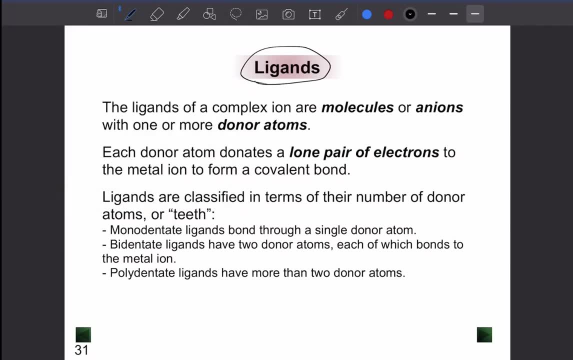 Octahedral is when you have a central single metal ion and there are six different ligands that are attached to it. Now let's go on to the topic of ligands. What are ligands? Ligands are molecules or anions With one or more donor atoms. 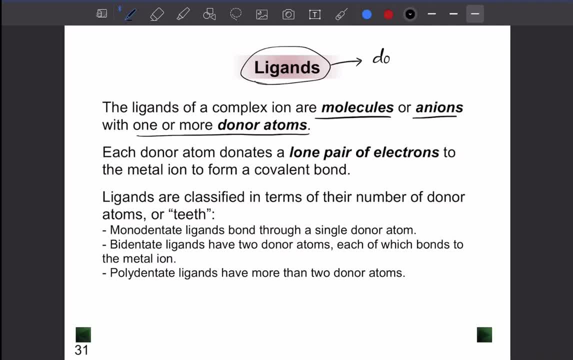 So one main characteristic of a ligand is it has donor atoms ready to donate electrons. So these are donor atoms that are ready to donate electrons. Each donor atom generally contains a lone pair of electrons to the metal ion and forms a covalent bond. 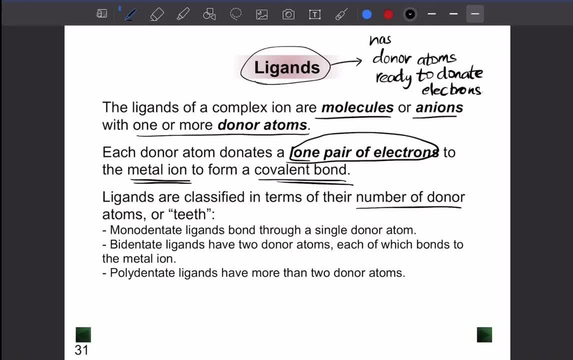 So ligands, in terms of the number of donor atoms or teeth, are classified based on them. So we have monodentate, bidentate and polydentate. So mono if it has one lone pair, Bidentate. sorry, let me write it this way. 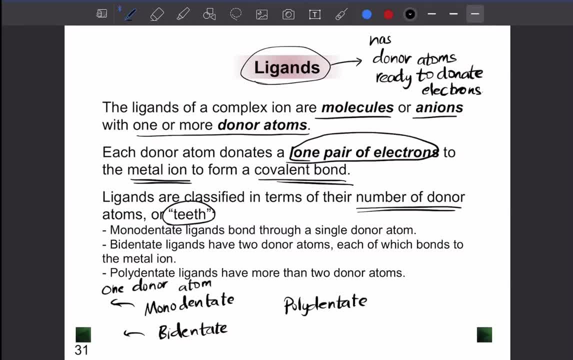 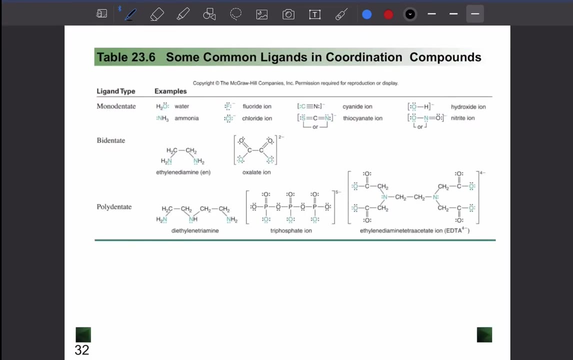 It has one donor atom, Bidentate if it has two donor atoms, Polydentate if it has more than two donor atoms. So let's see some examples of these ligands. So you have monodentate, bidentate and polydentate. 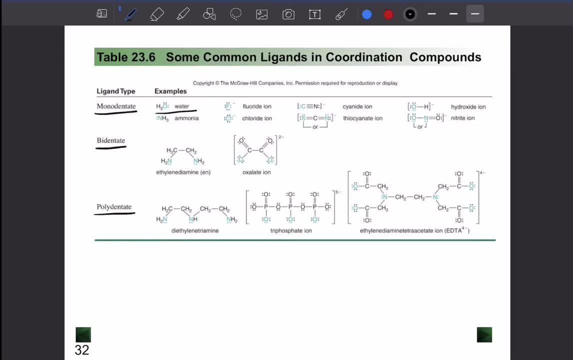 So the best example of monodentate ions is water. So water is an example of a monodentate ion, So it has the oxygen. So if you consider H2O, so you have oxygen connected to two hydrogens with two lone pairs. 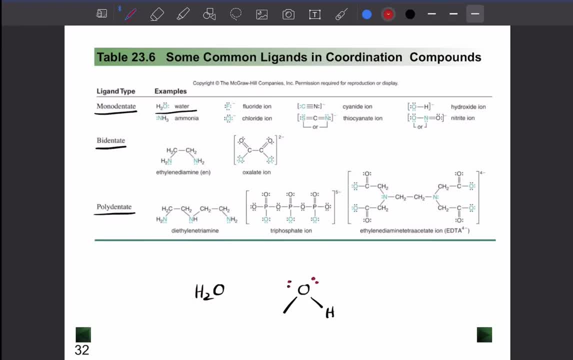 So the two lone pairs that are on oxygen, these two lone pairs can be donated. So because that's the reason why it becomes So because it has one donor atom. So we call this a monodentate ligand. Now there are elements where you have, even if you have a single compound, there might be multiple donor atoms. 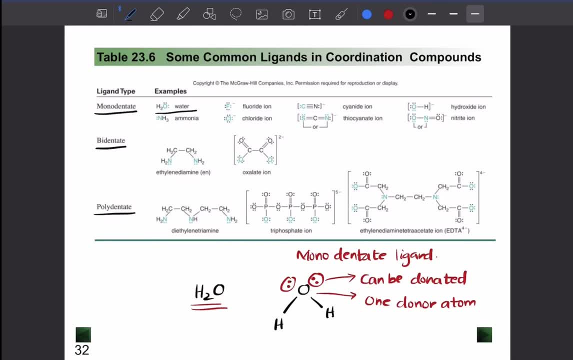 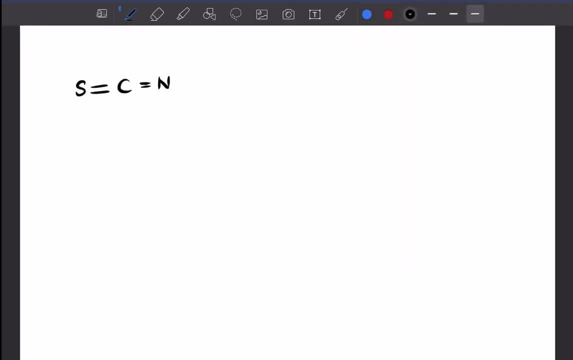 But they can only donate once. So what does that mean? So if you take an example of Thiocyanate- This is an example of thiocyanate- So if you take sulfur here and nitrogen here, There are two elements that have lone pairs of electrons. 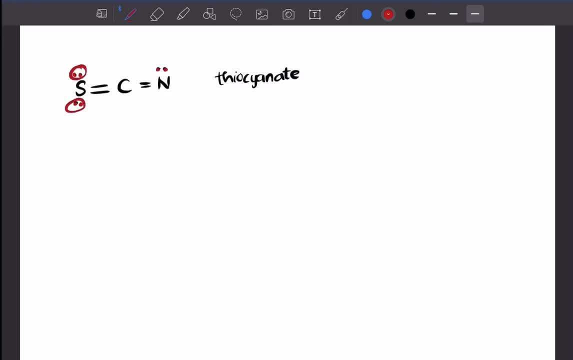 One is sulfur with two lone pairs and nitrogen with one lone pair. Now the chances are That either sulfur will donate or nitrogen will donate. Remember that it is either or, Which means that if one donates, The other does not donate. So these are also called monodentate ligands. 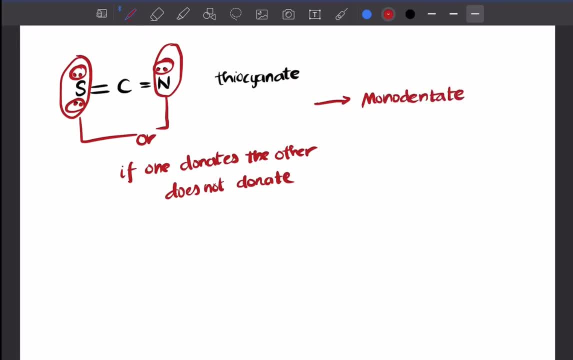 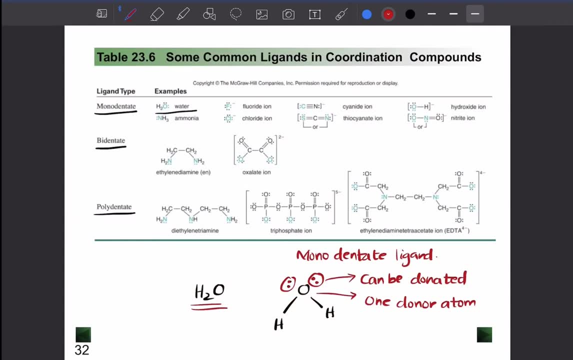 Because there is only one element at any given point of time That donates its electron pair to form the bond. So there are multiple elements like these. For example, One is thiocyanate ion, The other is nitrite ion, Which is NO2.. 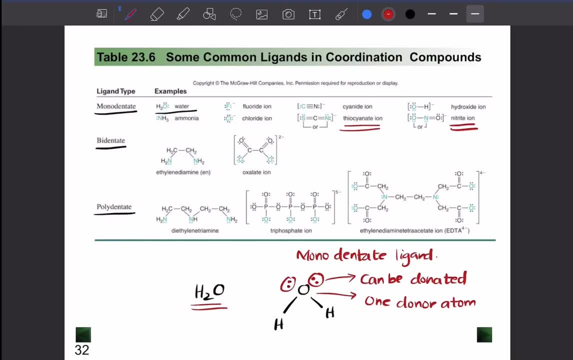 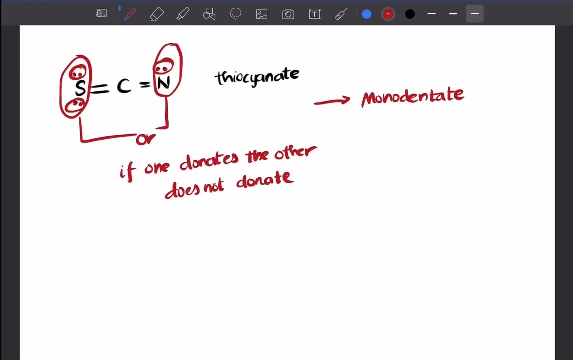 You also have Cyanate. You have hydroxide ion, Which is another example. Next, let's look at bidentate ions. So bidentate means there are Two donor atoms. One of the most common examples Is a compound called ethylene diamine. 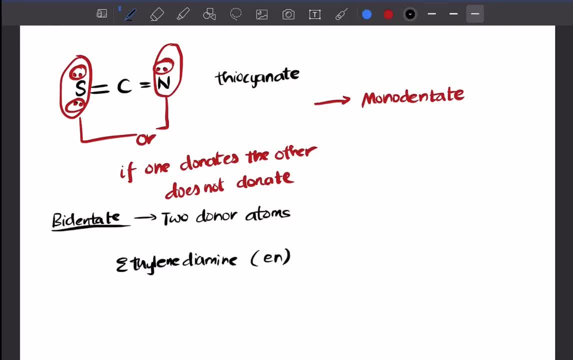 Or the short form is EN. So it's basically CH2.. Bond- CH2.. Bond NH2.. Bond- NH2.. So the nitrogen here, The nitrogens that are here, Each can donate its lone pair And form a bond. 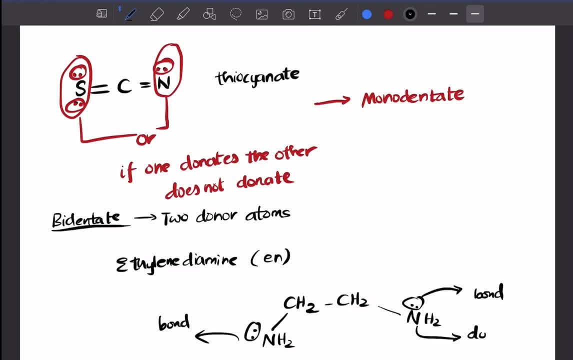 Right. So the nitrogen here Acts as a donor. Yet this nitrogen can also act as a donor And they can Both donate At the same time. So these elements Are called Bidentate ligands. So one of the examples: 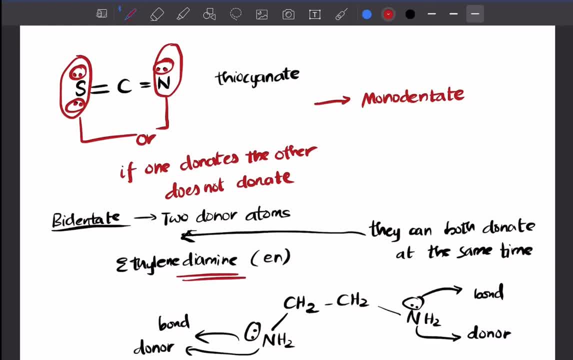 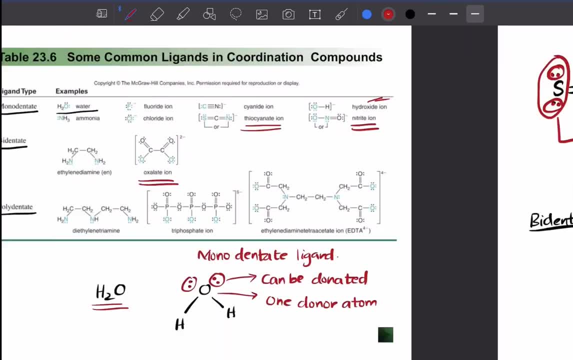 Is ethylene diamine, So written as the short form EN. The other example is an oxalate ion. Oxalate ion is C2O4 minus, O4, 2 minus. This is an example of another ion. So where you have two capons. 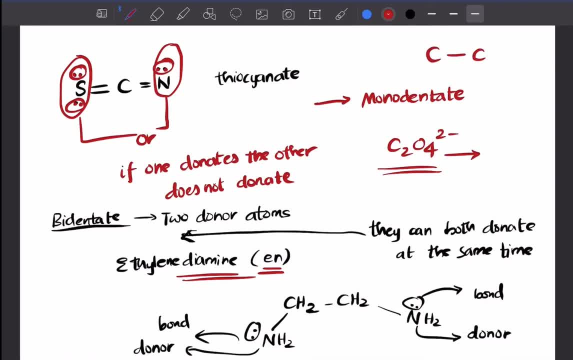 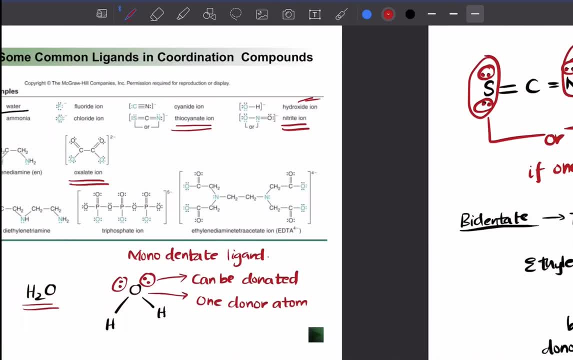 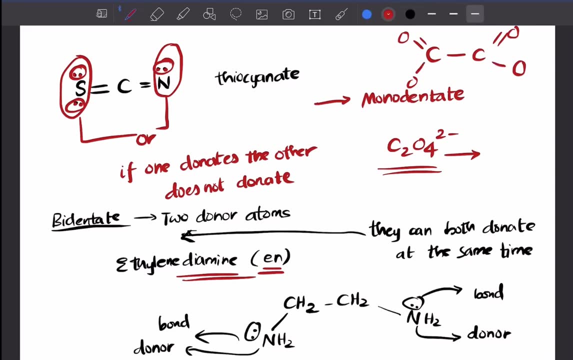 That are combined with oxygens. So this is an example of an oxalate ion And an oxalate ion. this is an example of an oxalate ion. Here these two oxygens are the ones that are ready to donate their electron pair, So this way this is also becoming a bidentate ion. 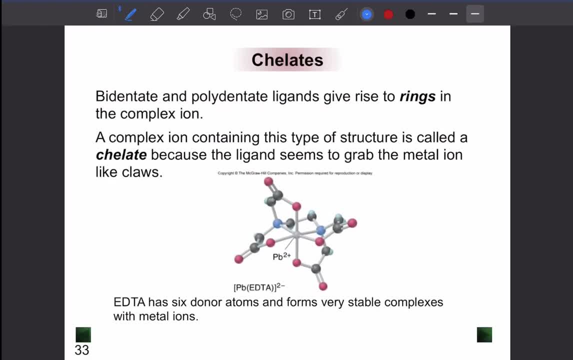 Next let us look at chelates, So bidentate compounds and polydentate compounds. because they bond to, they have more than one donor atom, they give rise to ring structures in the complex ion formation. So a complex ion containing this type of a structure is called as a chelate. 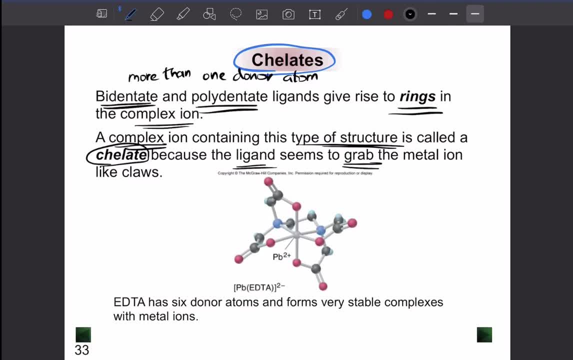 So because the ligand seems to grab the metal ion like cloths, so you basically have like a cloth structure, so bonding to the metal ion. So these types of elements are generally called chelates. So I am sorry we did not discuss polydentate. 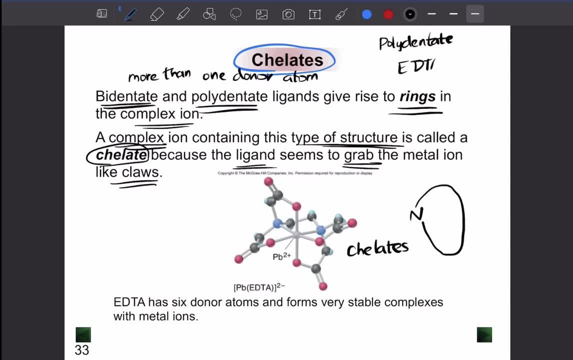 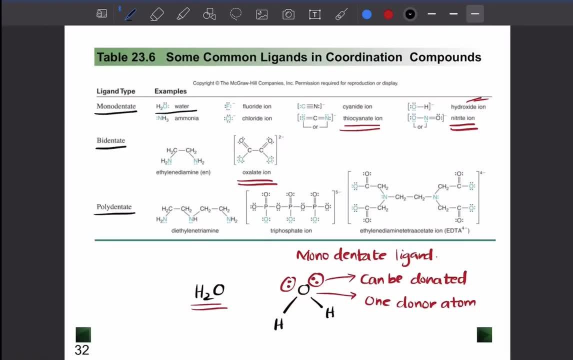 Polydentate. another example of that is EDTA, ethylene diamine, tetrahydroxylate acetic acid. So this is tetraacetate, ethylene diamine, tetraacetate ion or EDTA. 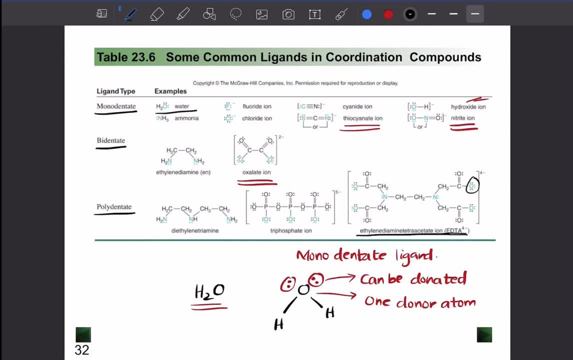 This is an example of a polydentate ion. So in EDTA there are six different elements that can act as donors. If you take a triphosphate, triphosphate has three different elements that can act as a donor atom, And another one is diethylene triamine. You have three nitrogens. that are ready to donate their electron pair. So this is a polydentate. So this is a polydentate. These are compounds that are generally called polydentate ions, So chelates are only formed when the ligands are either bi or poly. So either they are bi-dentate or polydentate. 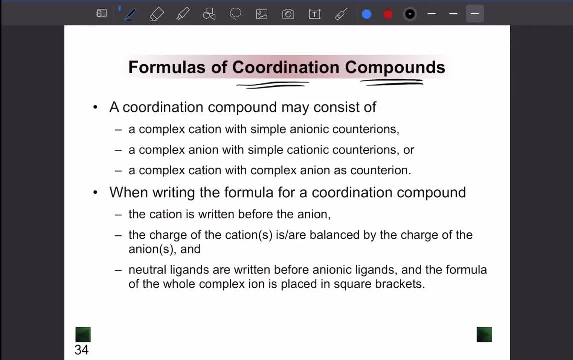 Now how do you write the formulas for coordination compounds? So a coordination compound can consist of a complex cation With a simple anionic counter ions, Or it can consist of a complex anion with simple cationic counterparts, Or a complex cation with a complex anion as the counter ion. So when writing the 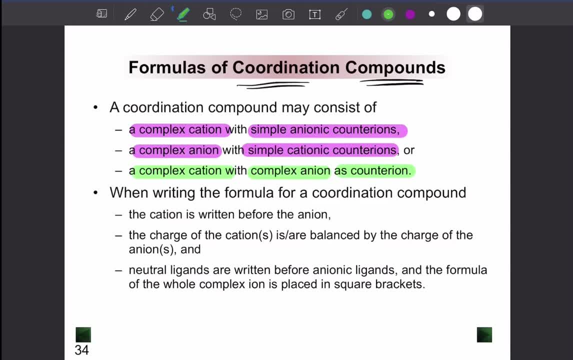 formula of a coordination compound. first thing to remember is that the cation is always written before the anion And the charge of the cation. we always have to balance it by the charge of the anion And if you have neutral ligands, they are. 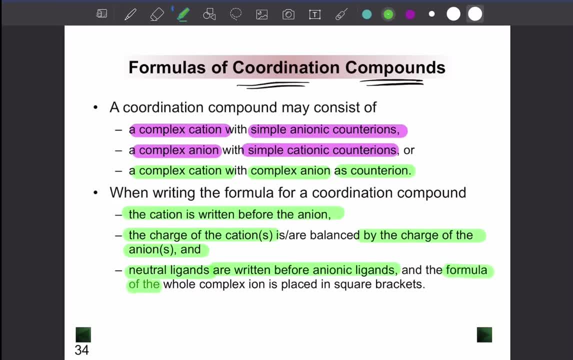 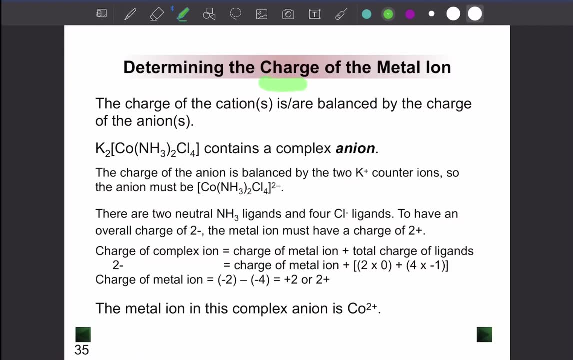 written before the anionic ligands, And the formula of the whole complex is placed in square brackets. So this is an example of how do you, what are the common rules that we use to write the formula? Now let's take an example. So how do you determine the charge? 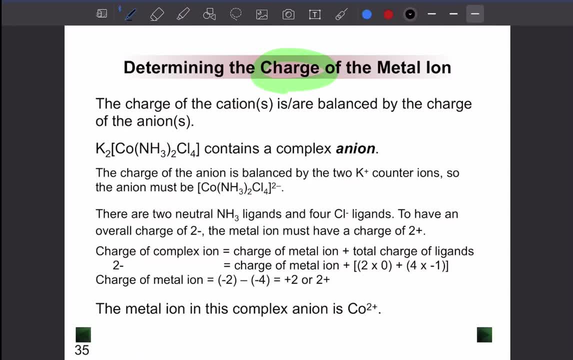 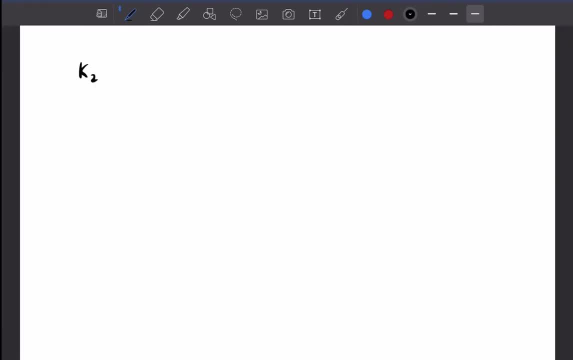 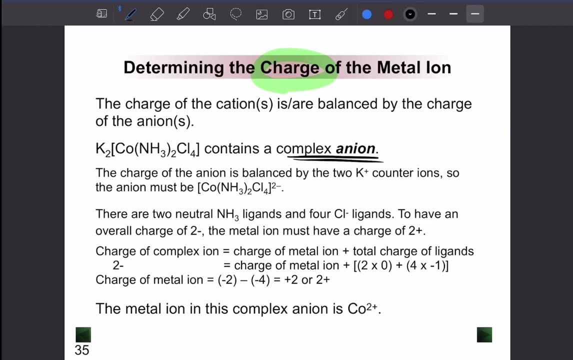 of the metal ion. So let's take a simple compound: K2.. K2.. K2.. K2.. K2.. C1.. C1.. NH3., NH3.. Taken twice, Cl4. Cl4.. So this is an example of a complex. So this is an example of a coordination compound. 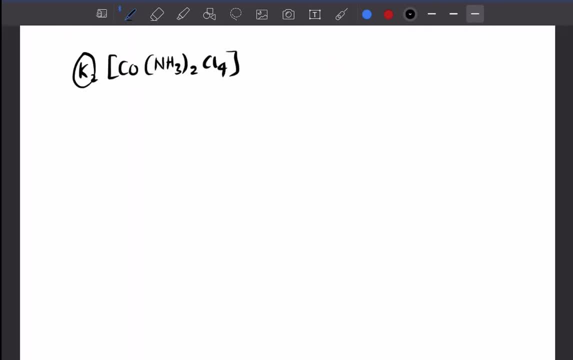 Now let's take the compound. We know that potassium is a cation, So this is the complex part. So this becomes the anion. So when it splits, when you mix it in water, you end up with 2k plus. 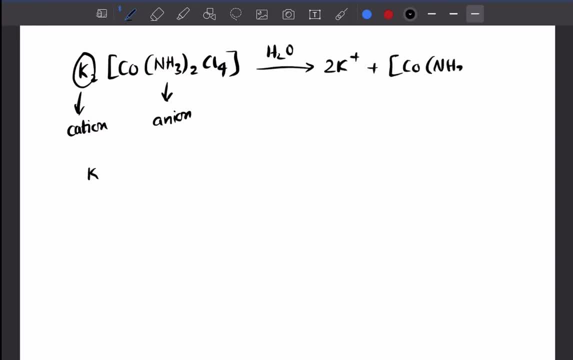 plus CO. NH3 taken to a Cl4 becomes 2 minus. So now you have a complex anion. So you have a complex anion. Now, by taking the complex anion into consideration, how do you calculate the charge? 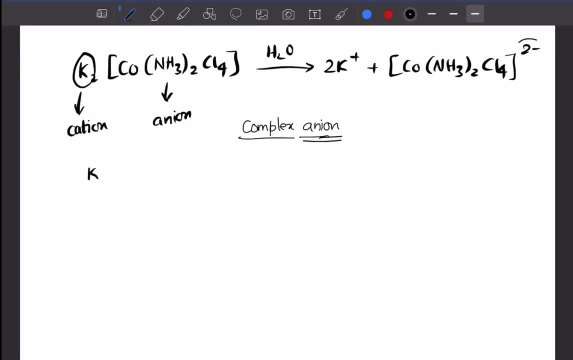 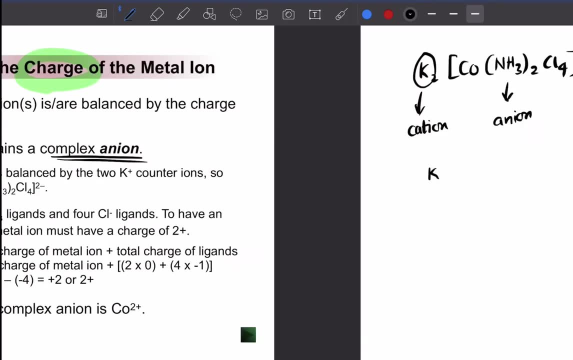 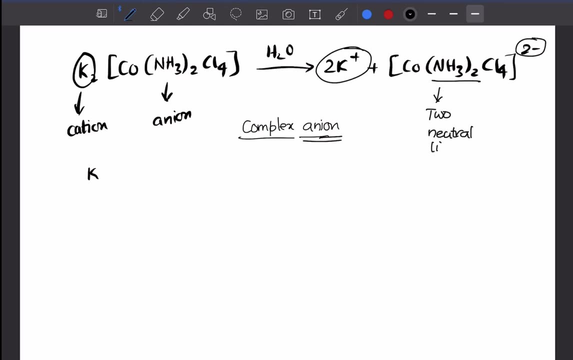 So we know that the anion itself has a charge of 2 minus because it has to counteract the positive cation. Now there are two neutral ligands. So the two neutral ligands are NH3s. NH3 is a neutral ligand. 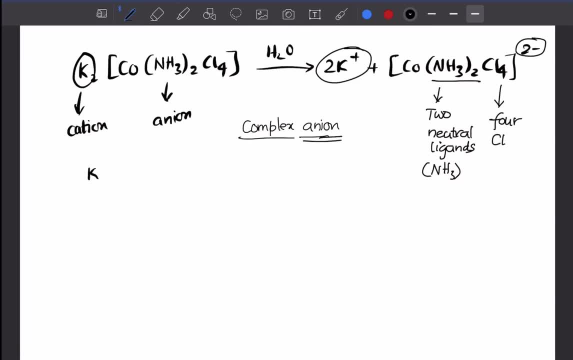 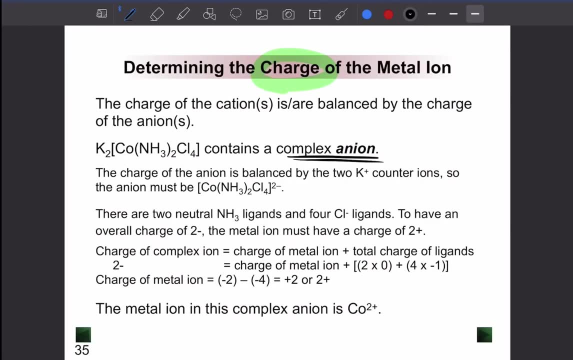 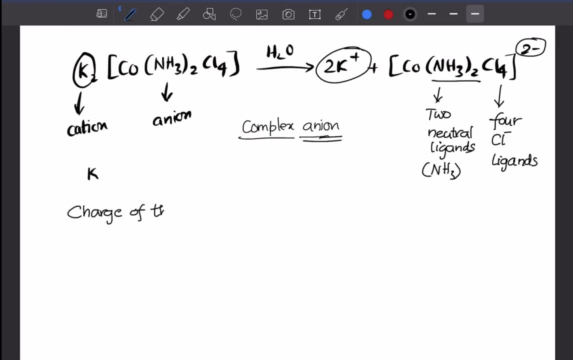 And there are four Cl minus ligands, So there are four Now, taking that into consideration. so what is the charge of the complex anion can be written as the charge of the metal ion plus the total charge. So we do not know the charge of the metal ion. 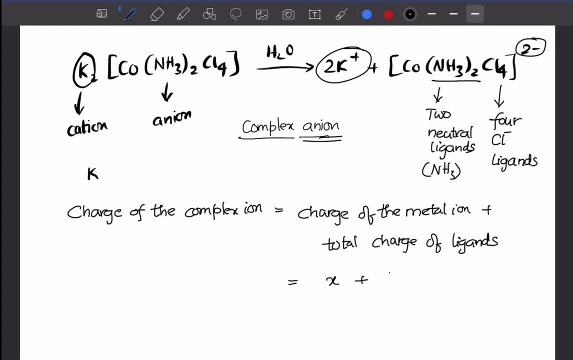 Let's call it EX. plus There are two different neutral atoms, So 2 into 0. plus you have four different chlorine atoms, So 4 into minus 1.. So the charge of the complex anion is already noted, which is negative 2.. 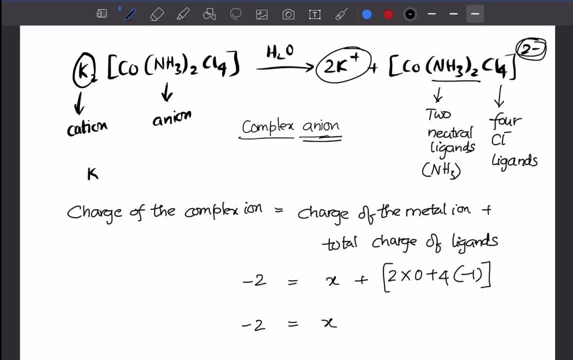 Now find EX, So it becomes minus 2 is equal to EX plus of minus 4.. So EX becomes minus 2.. So if minus 4 goes this side, so you have plus 4.. So you get a charge of plus 2.. 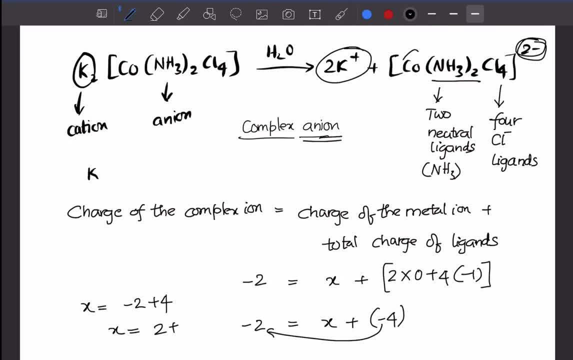 So you get a charge of plus 2.. So now we know the central metal ion here is cobalt. So cobalt here has a charge of 2 plus. So this is the central metal ion in this coordination compound. 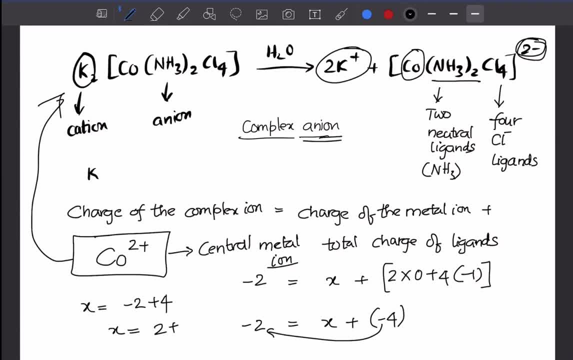 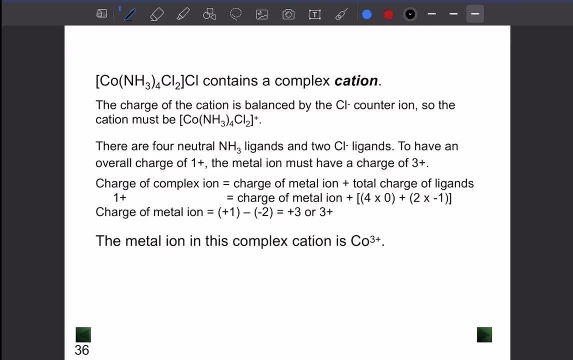 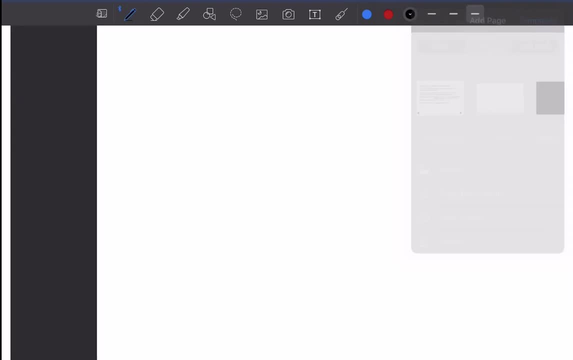 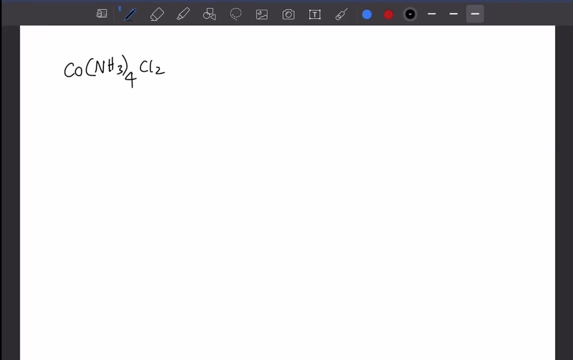 So this is how you can calculate the charge on the central metal ion Next. So let's try another one. You have C-O-N-H-3 taken 4, C-L-2 and C-L, So notice that we always write the cation first. 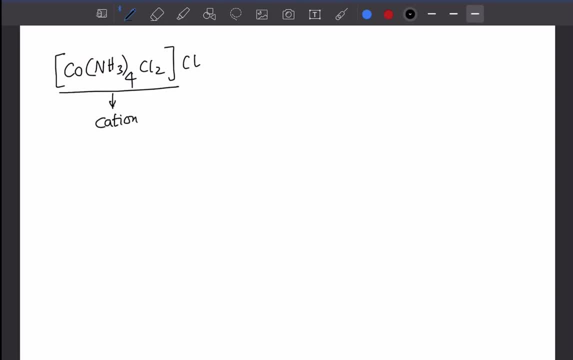 So this is the cation, So this is the anion. So here we have a complex cation And all of it are inside, So everything inside. So NH3. And CL are both ligands, Right. 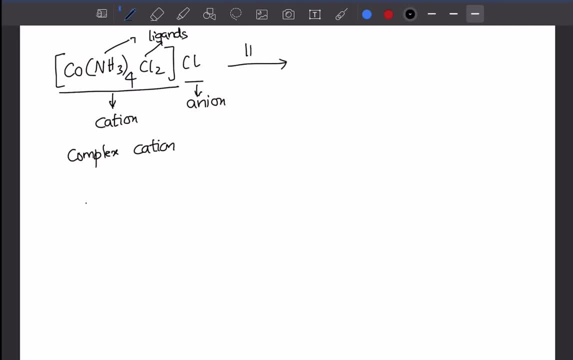 So you have. If you put it in water, You get C-O-N-H-3 taken 4, C-L-2 plus CL- So because there is one minus, it becomes plus. So the complex cation that we have is C-O-N-H-3 taken 4, C-L-2 plus. 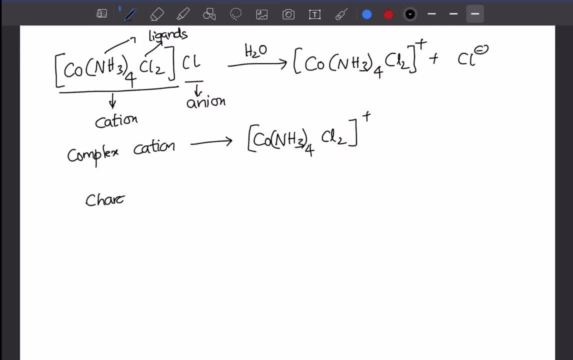 Now use the same formula. So which is the charge of the complex ion? is the sum of the charge of the metal ion plus the total charge of the ligands. Now, what is the charge of the metal ion? So the charge of the metal ion here? we do not know that, So let us call it x, So let us take the total charge of the ligands. 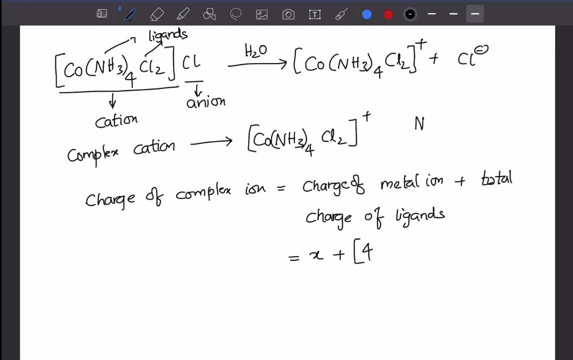 So there are four neutral ligands. So NH3 here is the neutral ligand. Cl is the charged ligand, So it has a charge Minus 1.. So there are two of them, So it becomes 4 times 0 plus 2 times minus 1 is equal to plus 1.. So the complex ion charge is plus 1.. 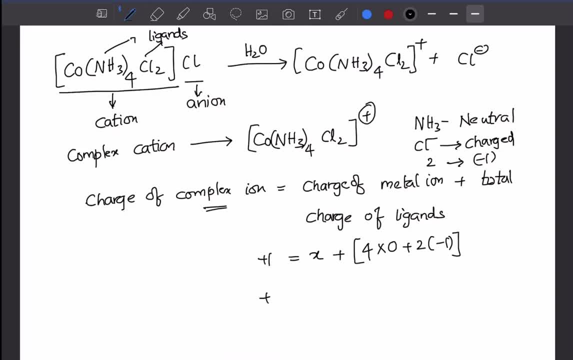 So we use that plus 1 here. So now plus 1 is equal to x minus 2. So x becomes plus 1 plus 2. So you get plus 3.. So the central metal, ion cobalt, has a charge of 3 plus So in this coordination compound 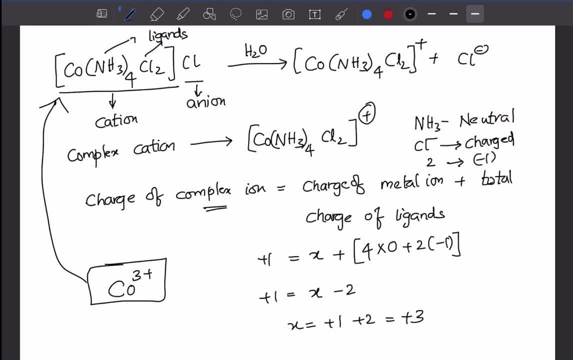 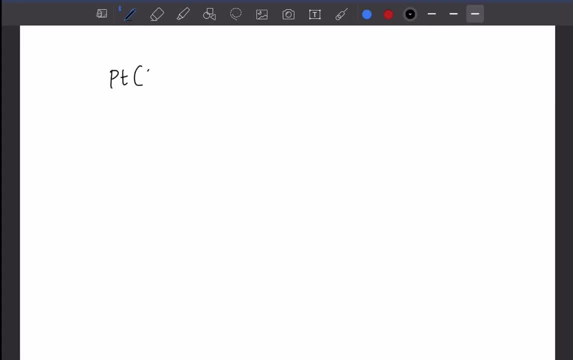 the central metal ion has a charge of 3 plus Now. so take another example of platinum. So now NH3 taken twice Cl taken twice Cl2.. So now here, calculate the charge of the platinum. So pause the video right here and try to solve this problem and calculate the. 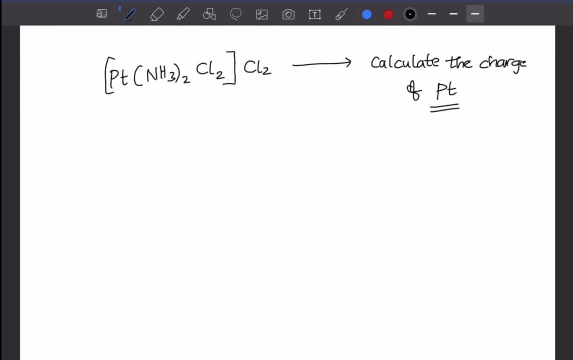 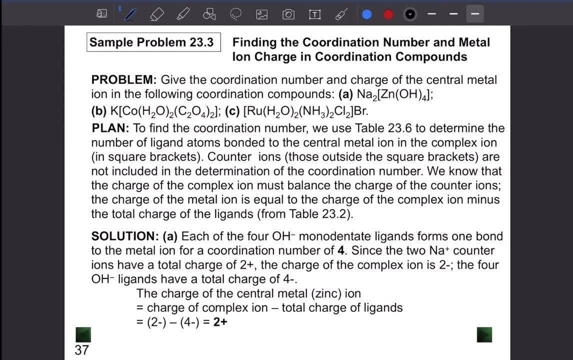 charge of the platinum metal. So also take a pause in this slide as well. You also have sodium, You have these three compounds. So try and answer and try to find these three compounds, The central metal ions charge, And also find the coordination number. So also remember that coordination number is the number. 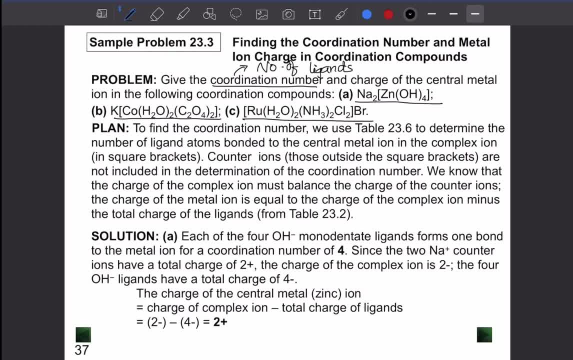 of ligands, So I'll do one of them. For example, in this, if you take the square brackets, everything inside it is connected to the metal is a ligand. So here OH is a ligand. There are four of them, So there are four ligands, So the coordination number is 4.. 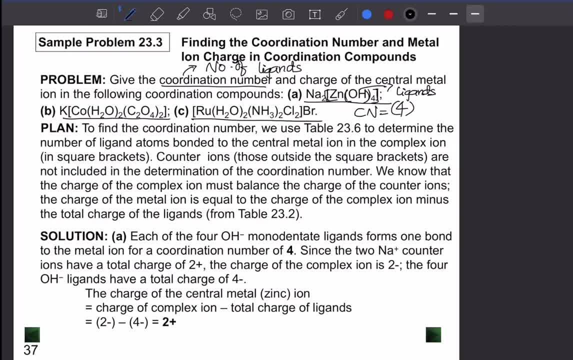 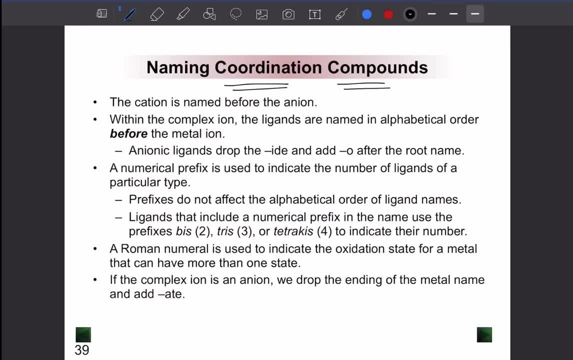 Now in this way, try for B and C. How do you name coordination compounds? So the cation is named always before the anion. Within the complex ion, the ligands are named in alphabetical order before the metal ion. So this is within the complex ion. 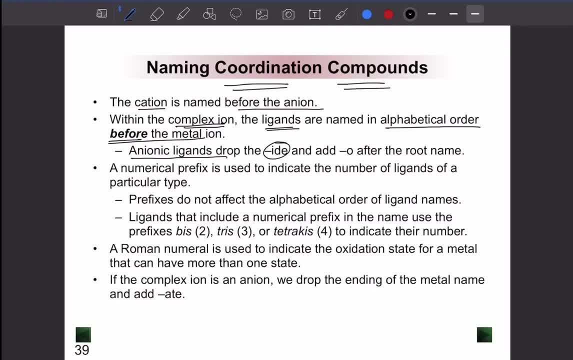 If you have an anionic ligand, we drop the IED and we'll write O at the after the root name. A numerical prefix is used to indicate the number of ligands of a particular type, So prefixes are used to indicate the number of ligands of a particular type. 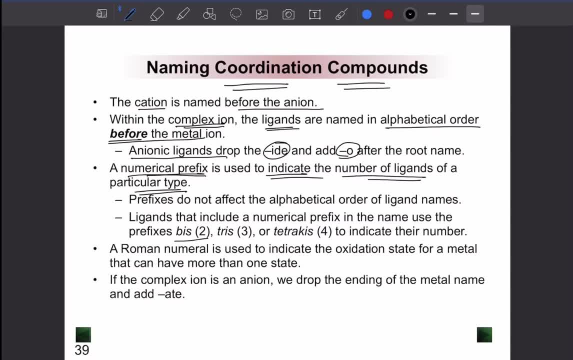 So prefixes do not affect the alphabetical order. So it can be bis, tris or tetrachis. If you have two of them, it's bis, 3, tris, 4, tetrachis. Now a Roman numeral is used to indicate the oxidation state of the metal that can have more than one state. 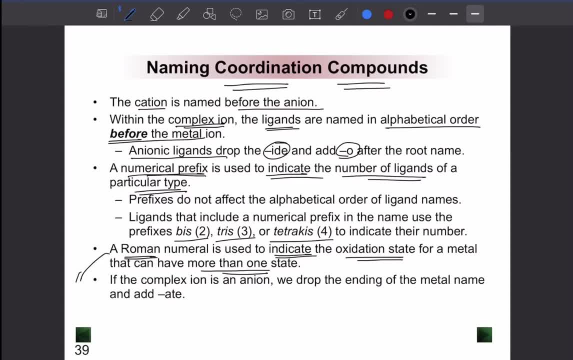 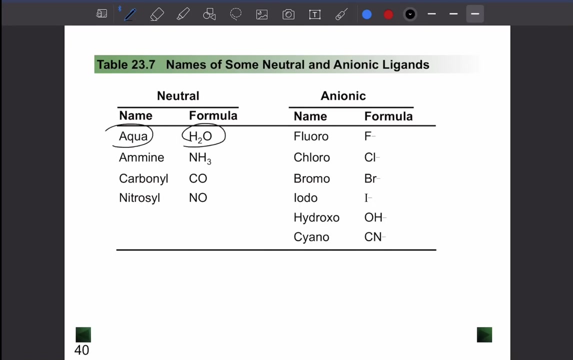 If you have only used this when the transition metal and the transition element, it has multiple oxidation states. Next, if the complex ion is an anion, we'll drop the ending of the metal and we'll write A. So an example of that would be: if you take H2O, we write AQUA. 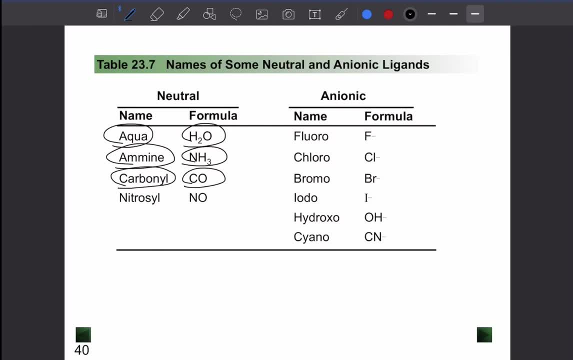 NH3 is written amine, CO is written as carbonyl, NO is written as nitrosyl F, fluoro. So IED becomes oro, Chlorine becomes chloro, Bromine becomes bloro. You have, OH becomes hydroxy. 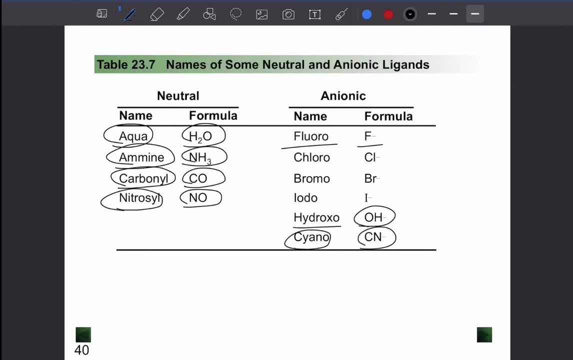 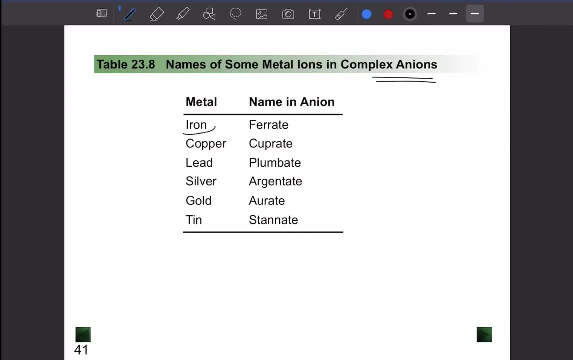 CN becomes cyano. So these are the common anionic ligand names and neutral ligand names. Next, for the metal complex anionic metals, the metal ions: iron is written as ferrate, Copper is written as cuprate. Lead is written as plumbate. 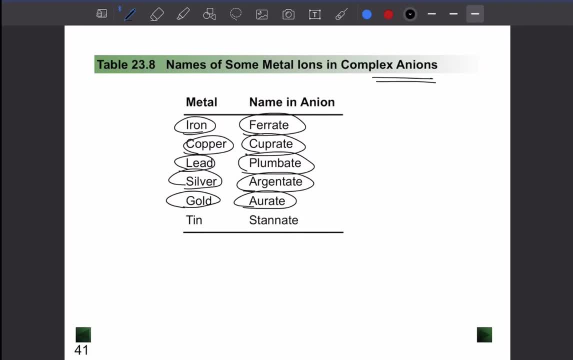 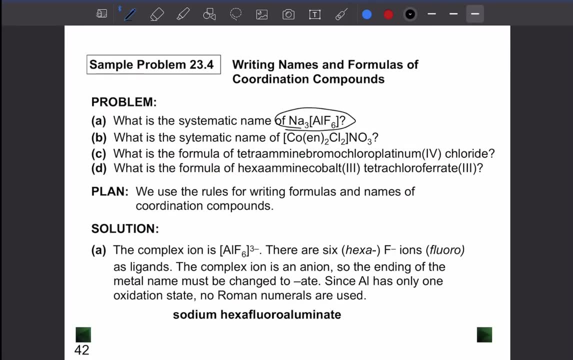 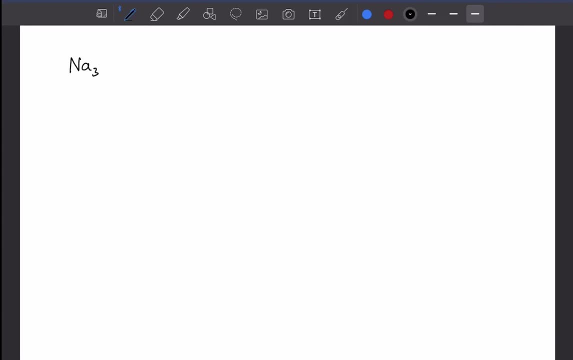 Silver is written as argentate, Gold as aurate, Tin as tannate. So let's try the first example: NH3, ALF6.. So the first rule is: cation is named before the anion. So here we know that sodium is the cation. 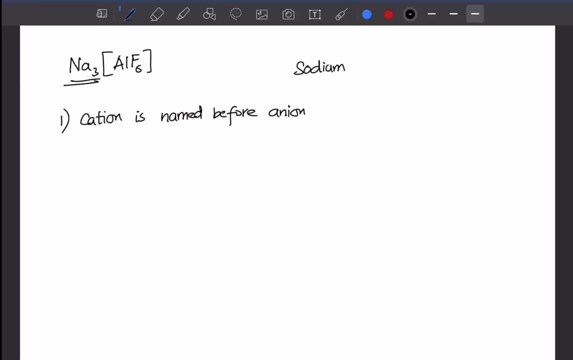 So the first name comes sodium. So we have a fluoride ligand. Next, inside the ligand name, we write the first ligand name. So what are the ligand names? So you have a fluoride ligand. 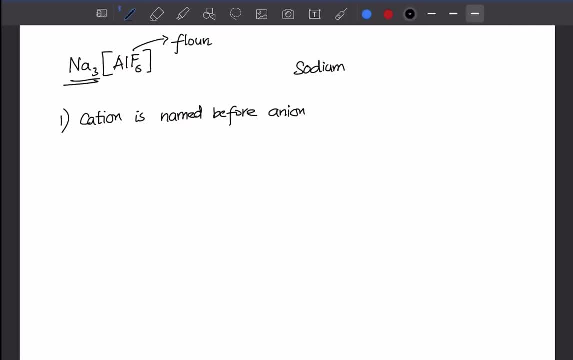 So you have a fluorine ligand, So we will remove fluorine and we will write fluoro. But there are six of them, So we can write hexafluoro. And there is aluminium- is the metal, So we remove fluorine. 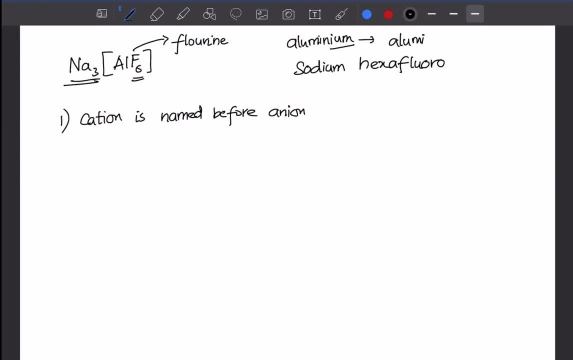 We remove em and we write 8.. So it becomes aluminate. So it becomes sodium hexafluoroaluminate. So this is the name of the compound here. Here I am not going to write the oxidation state for sodium, because sodium has a fixed oxidation state. 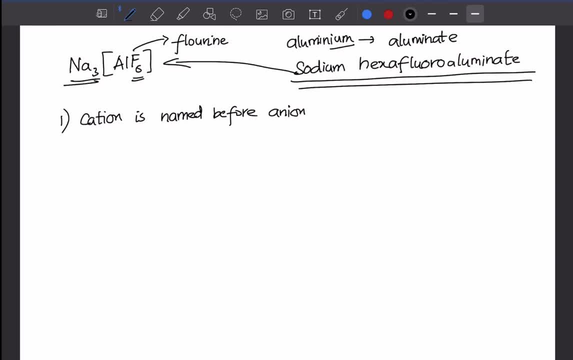 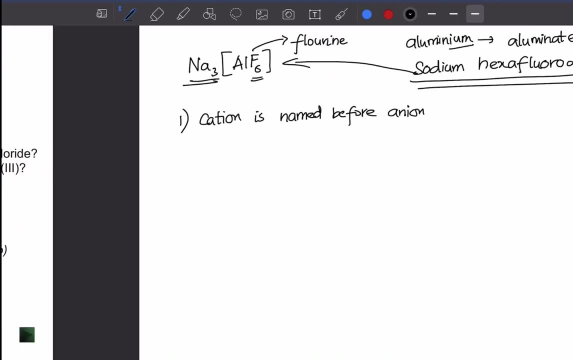 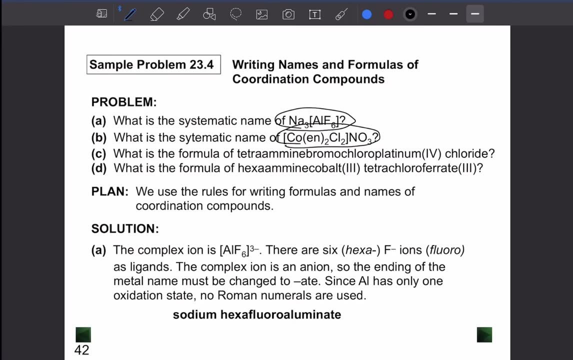 So aluminium has a fixed oxidation state of plus 3.. So there is nothing more than that, So we can write simply that name. Next, let's try another one, Which is COEN, taken twice Cl2, NO3.. 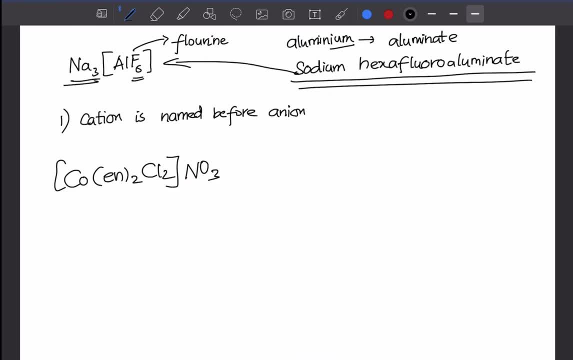 So this is the compound that is given. Now we know that this is the anion and this is the cation, So always we name the cation first. Now, in terms of the cation, we have cobalt. 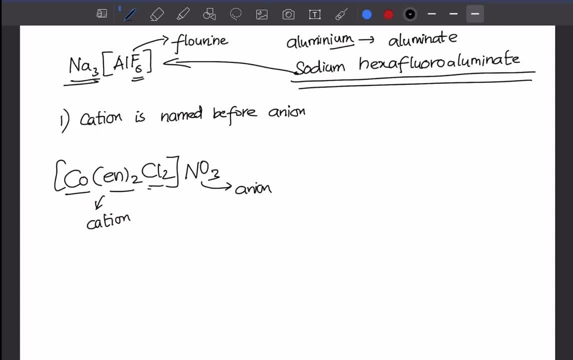 We have ethylenediamine and we have Cl2.. Notice that EN represents ethylenediamine. Now let's start, based on the alphabetical order. We have two ligands: We have chlorine and we have ethylenediamine. 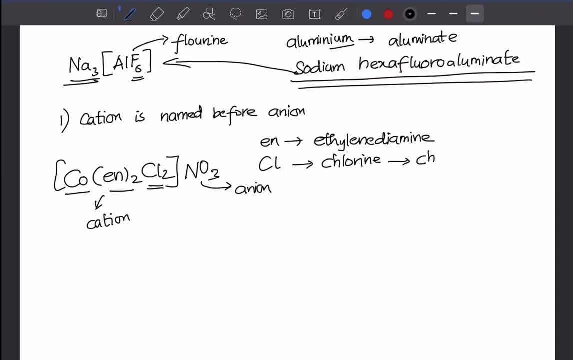 So chlorine will end up being written as chloro. So let's start with alphabetical order: chloro: There are two of them, So we write dichloro. And there are two ethylenediamines, So we cannot write dienamine. 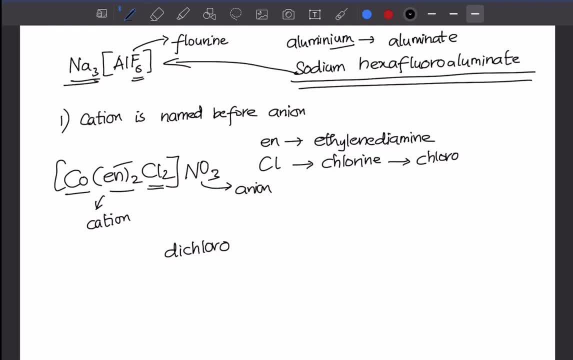 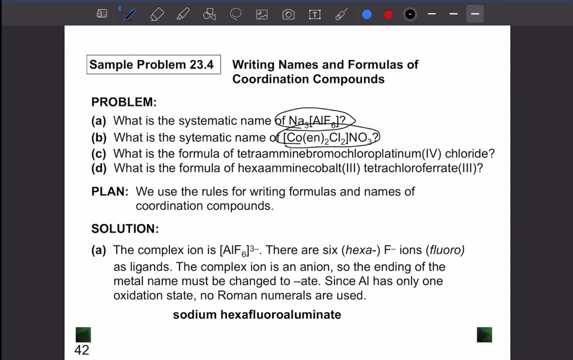 So diethylenediamine, So we write it as bis, So bis, And in brackets write down ethylenediamine, So you have cobalt. So that's the compound that you have. 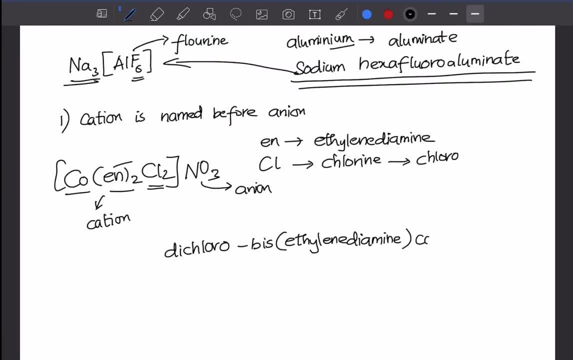 So use the cobalt here. But we know that cobalt has multiple oxidation state. We want to know the oxidation state for cobalt. Now let's check each of them. We notice that ethylenediamine is neutral. 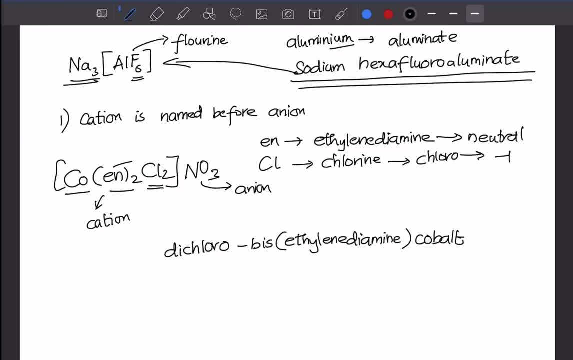 Chlorine has a charge of negative 1.. So now we know that the metal has a charge of positive 1, because NO3 has minus 1. So it becomes plus 1.. So plus 1 is equal to 0.. 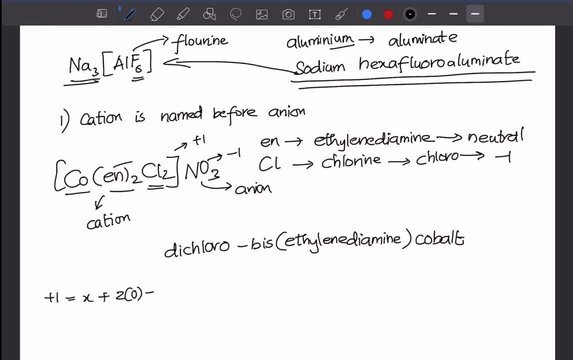 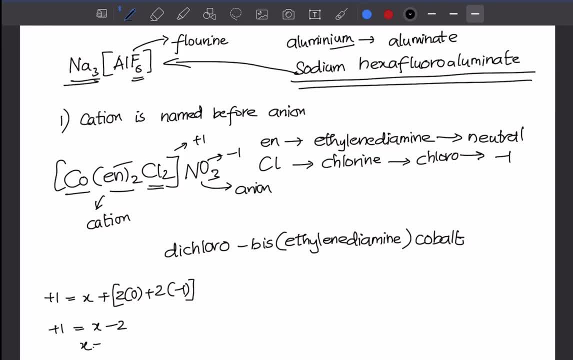 So it becomes: X minus 2 is equal to plus 1. So X becomes plus 1 plus 3. So plus 1 plus 2. So it becomes plus 3. So the cobalt here has 3 plus charge. 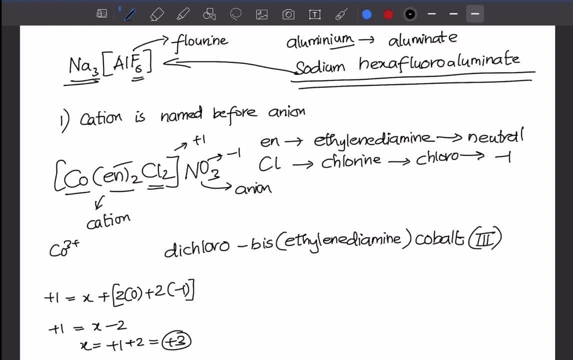 So we write cobalt 3.. And we have NO3 here, So we write nitrate. So this is the name for the final compound. you have to write the hyphen here, so dichlorobisethyldiamine. 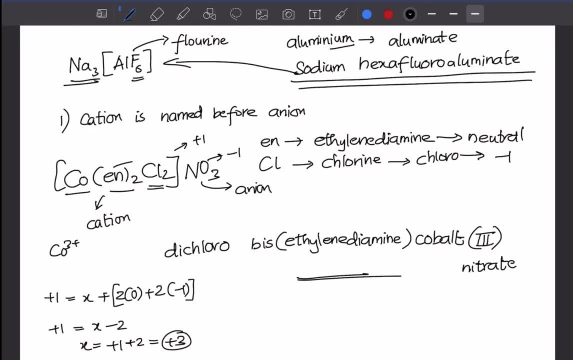 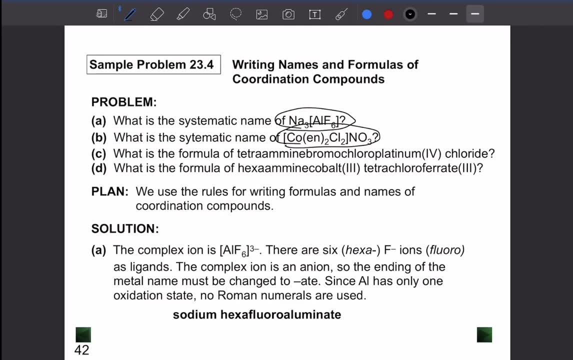 cobalt 3 nitrate. so this is the compound that you end up with next. so in the next one, they have given you tetraamine bromochloroplatinum 4 chloride and you have hexamine tetrachloroferrate. 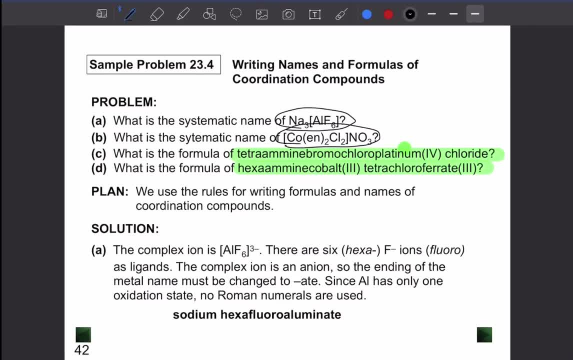 now I will do one of them, so you try the other one at home. so let me do C now. always write the cation before the anion. so the anion is chloride. so let us write Cl, right, and it has an oxidation state of 4, we do not know the total ions. 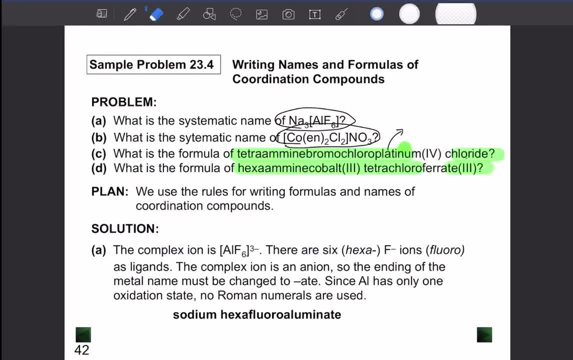 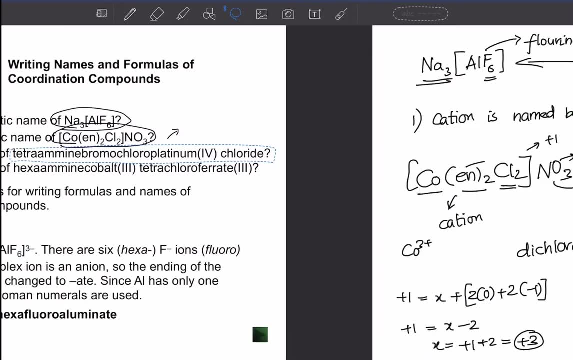 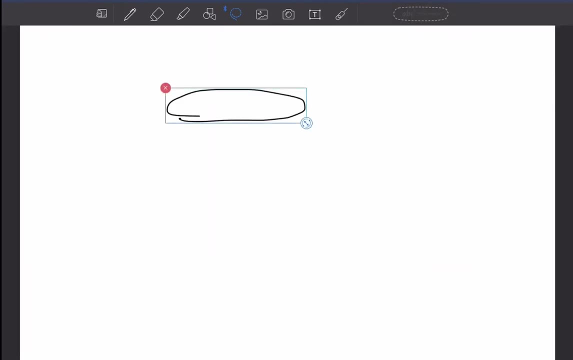 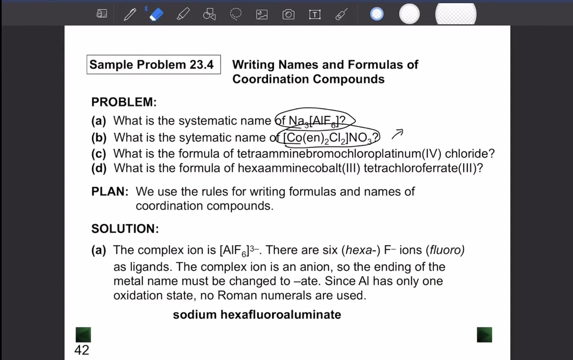 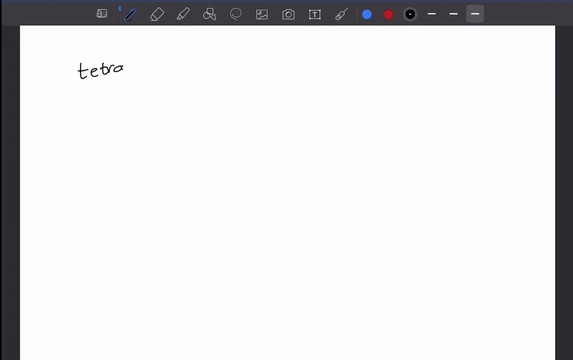 It has an oxidation state. do not write that right now, so do not write anything right now, so let me write the compound separately. So you have tetraamine bromochloroplatinum 4, 4 tetrachloroplatinum 4 chloride. so this: 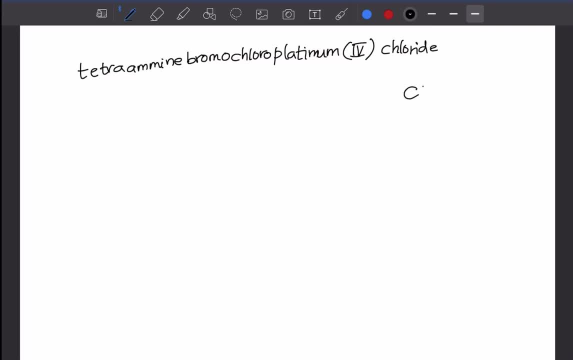 is the name given. So we know that The outside one is fluoride and there is bromine, there is chlorine and there is one of each and there is tetraamine, so NH3, there are four of them and platinum is the. 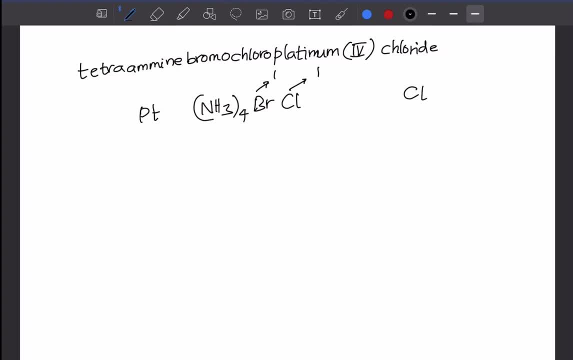 metal. Now we can write that based on the adder. we have platinum NH3 taken 4 BrCl, so this is the complex anion. and chlorine- here Cl- is the complex anion. Here this becomes the complex cation.